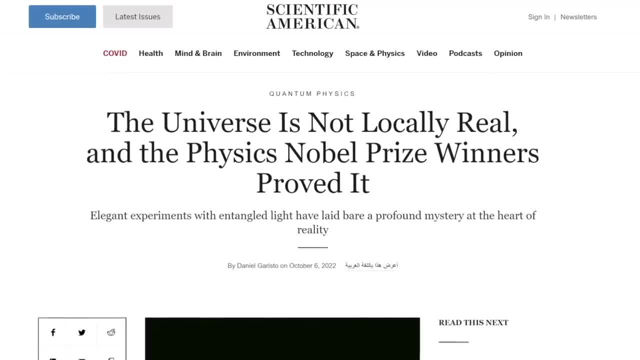 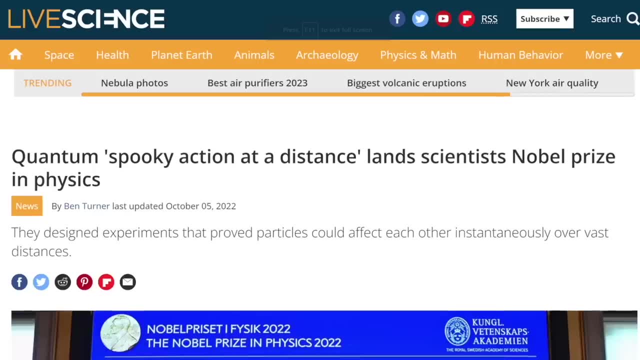 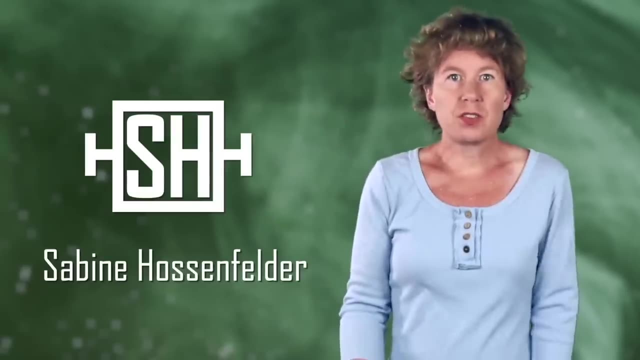 According to the headlines, last year's Nobel Prize in Physics was awarded for showing that the universe is not locally real, Or for spooky quantum behavior and spooky action at a distance, Or for exploring quantum weirdness. What's that supposed to mean? Is the universe really not locally real? 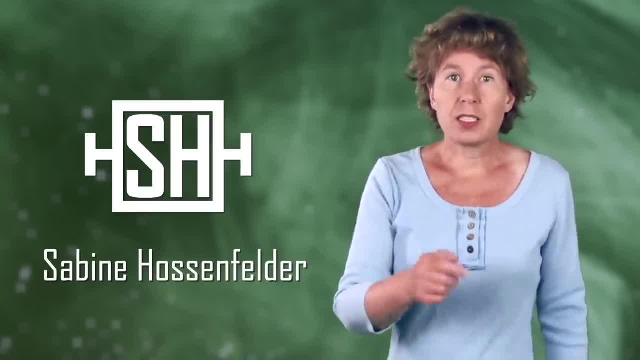 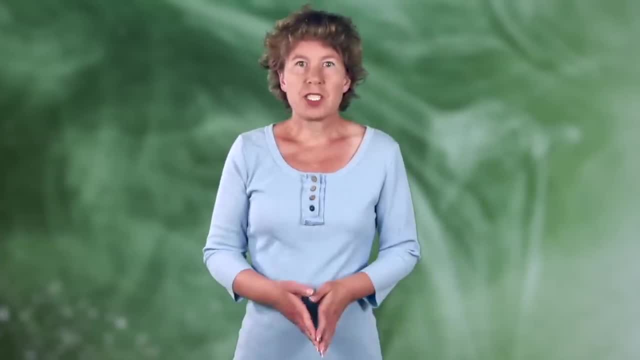 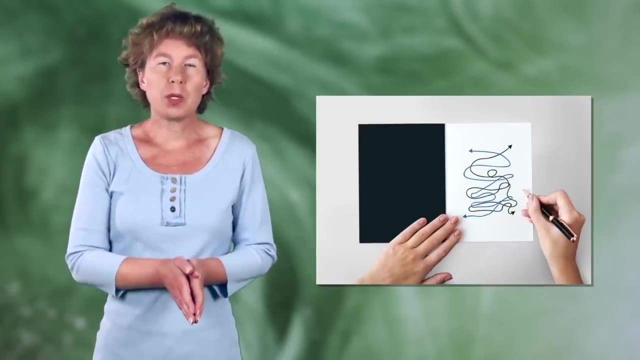 or not really local or not really real. That's what we'll talk about today. My grad plan for this video is that we'll first look at what locality means, then we'll talk about quantum mechanics and then we'll combine both. Let's start with locality. 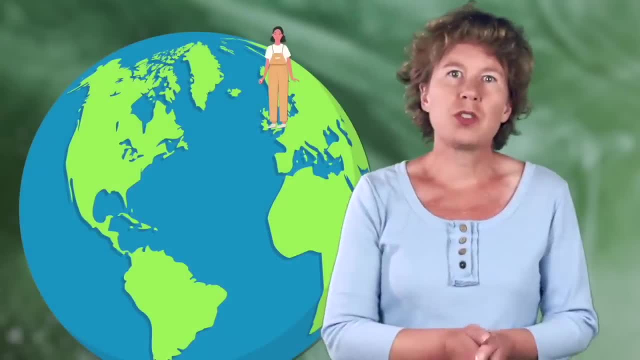 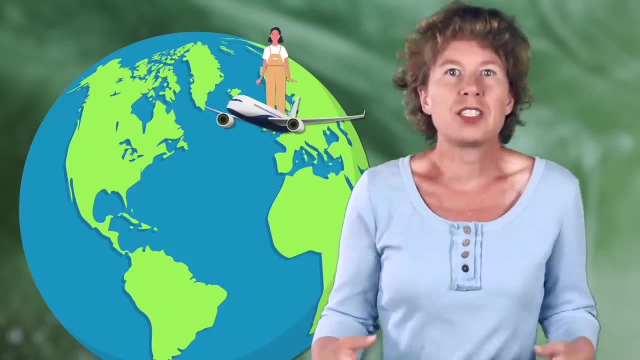 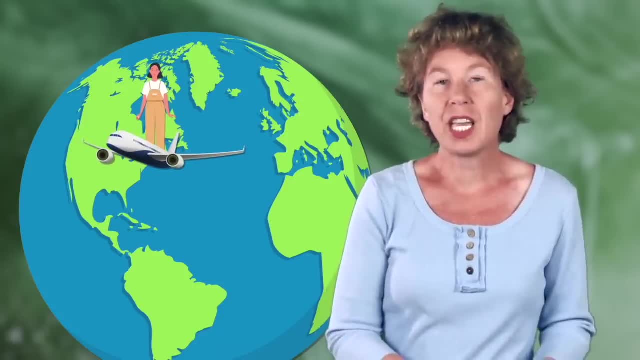 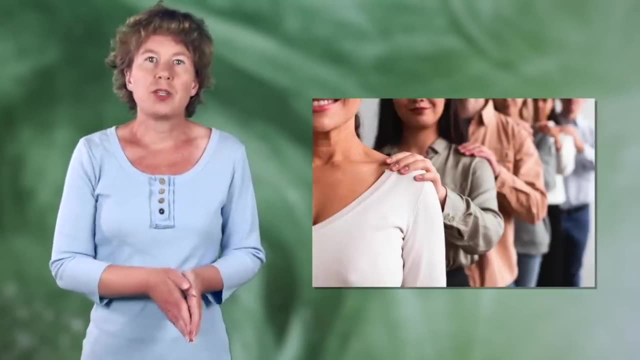 queue and then drag yourself into the immigration queue and then drag yourself into the immigration queue. There's no instantaneous going anywhere. It's not just travel, it's generally any interaction. You can only act on things next to you, And it's not just you. No, really, I swear. 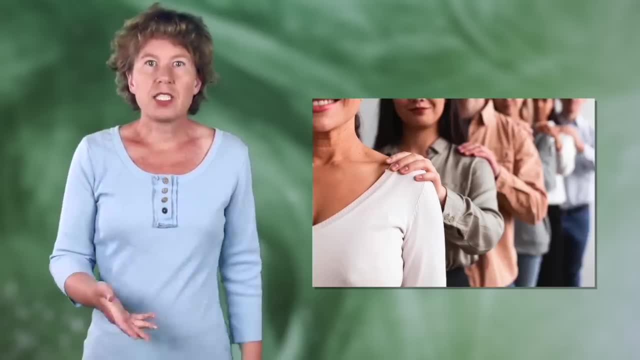 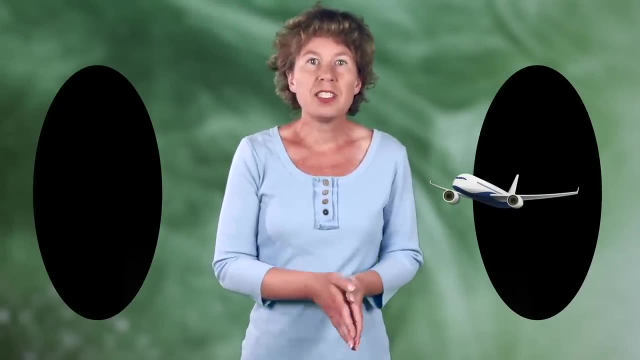 Anything can only interact with things right next to it. This is what we mean by locality. Non-locality would basically be a portal. Something goes in and instantaneously appears as where. Now, if you could travel non-locally, that might allow you to go. 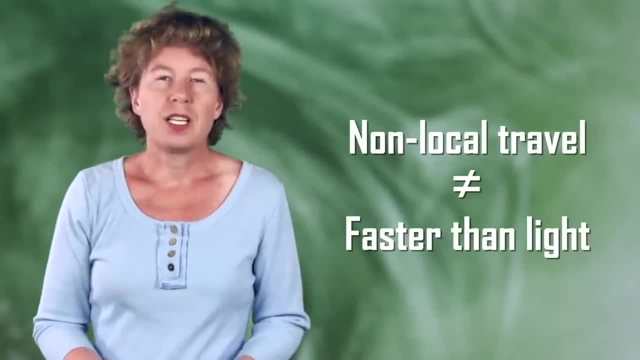 faster than light, But it doesn't necessarily have to. Alice could go to Tokyo faster than light without taking a portal. Bob could go through a lame portal that brings him to New York even later than Air France and leaves his bag in Paris again. 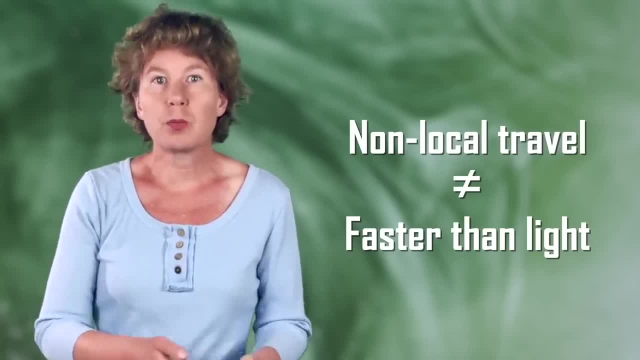 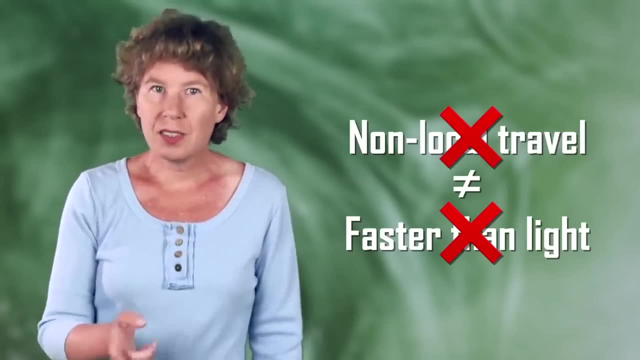 So non-locality and faster than light travel are two separate things, But the two are related in that Expedia isn't offering either. Maybe more importantly, though not unrelatedly, neither of them is allowed in Einstein's theories of space and time. Yes, that guy. 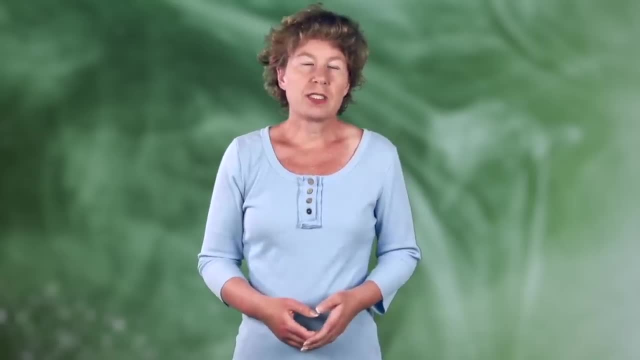 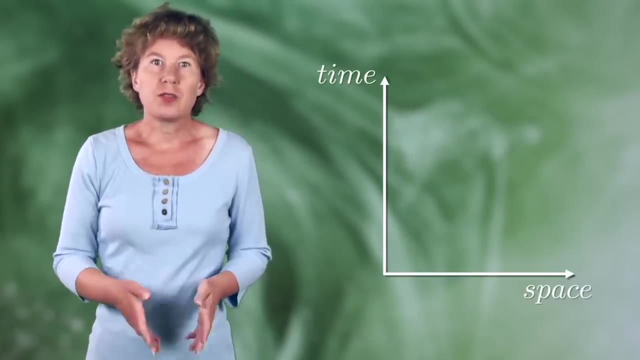 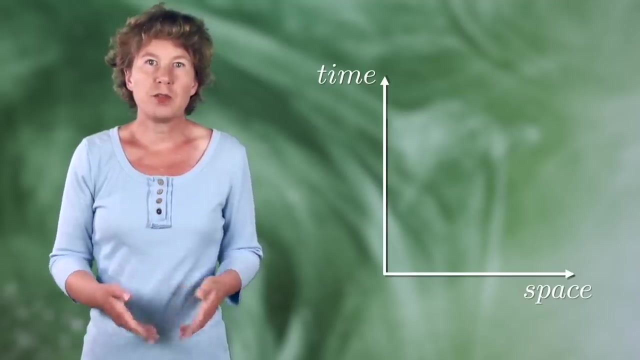 again. We can make a little drawing to see what this means. This is a space-time diagram. The horizontal axis is one dimension of space, say left or right. The vertical axis is time. If you don't move but sit still, that's described by a vertical line in this diagram. If you 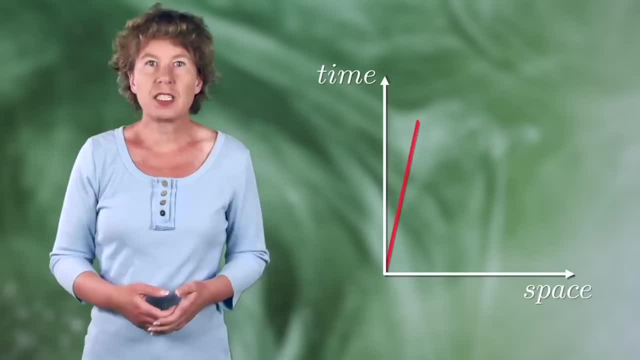 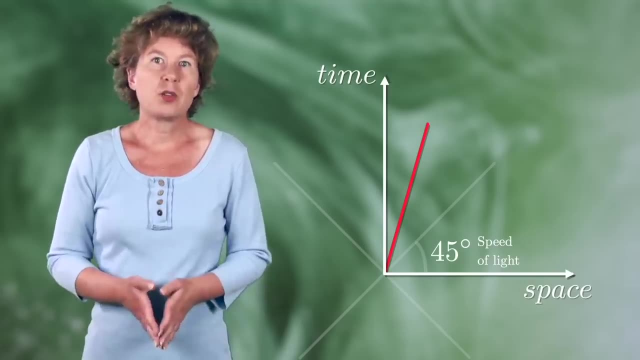 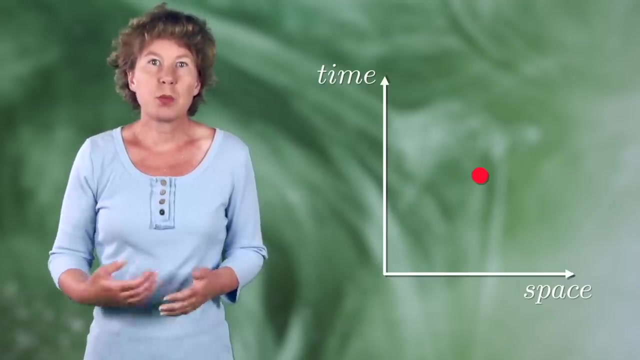 move at a constant velocity that makes a line at a fixed angle. By convention, a 45 degree angle is the speed of light. According to Einstein, nothing can go faster than light. This means if an event happens here, then anything that can be influenced by this event must lie within a region that's. 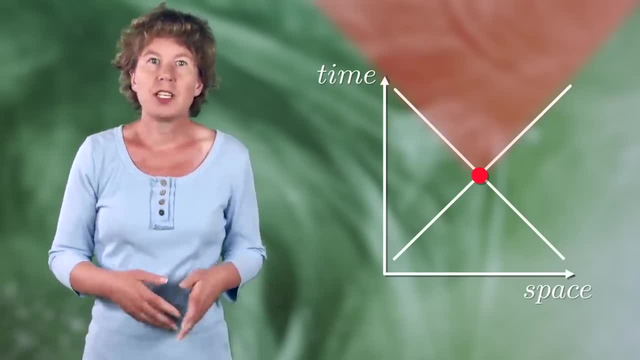 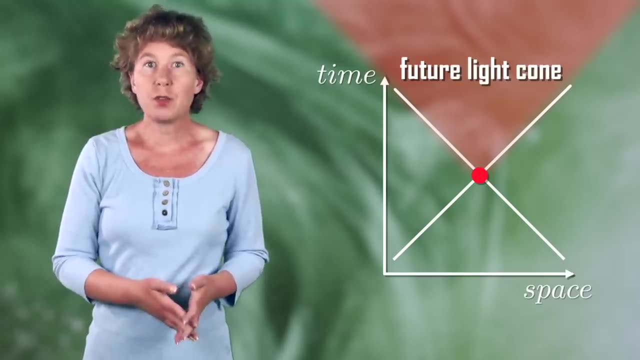 bounded by 45 degree lines emerging from the event. This boundary is called the future light cone, and the region that can be influenced from the event is that inside the future light cone, Likewise, there's a region which contains everything that can influence the event, which is the inside. of the past light cone. If something could go faster than the speed of light, it could enter your light cone like this, And if nonlocality was possible, it wouldn't have to respect those light cones either. It could just jump into your light cone. 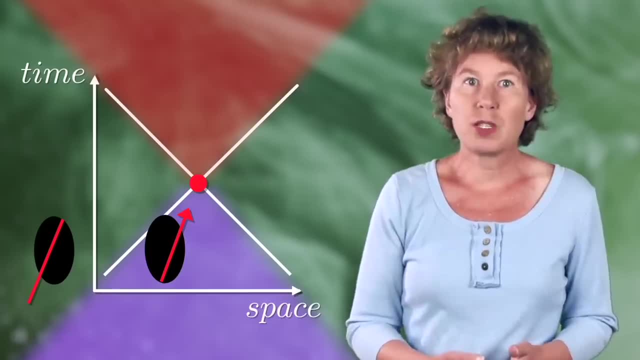 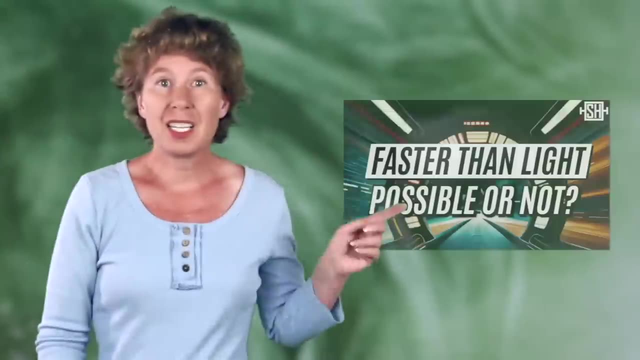 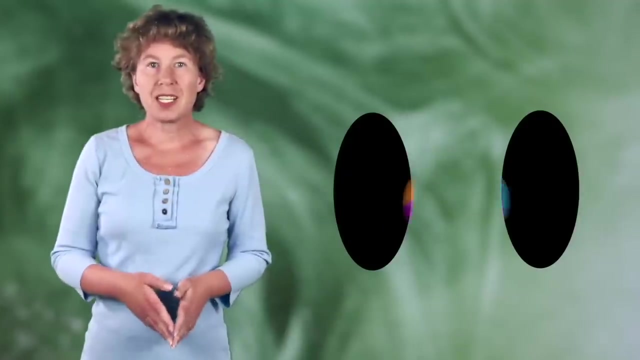 For the rest of this video, we'll assume that faster-than-light travel can't happen and just look at nonlocality. If you'd rather hear me talk about faster-than-light travel, I have another video on that. This video suggests that reality is local in that these jumps in space-time don't. 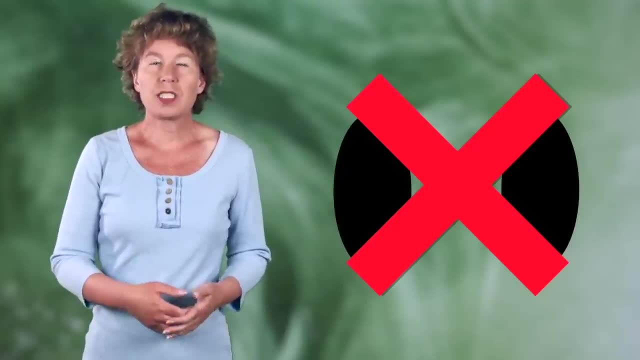 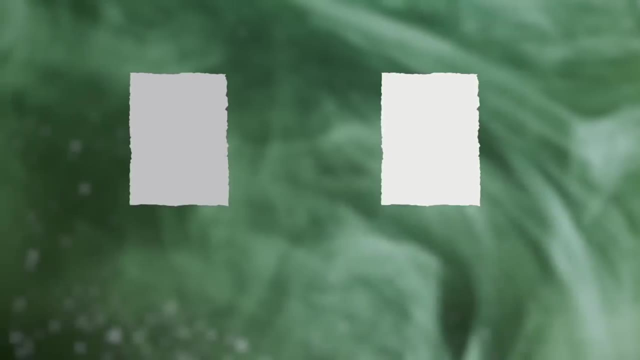 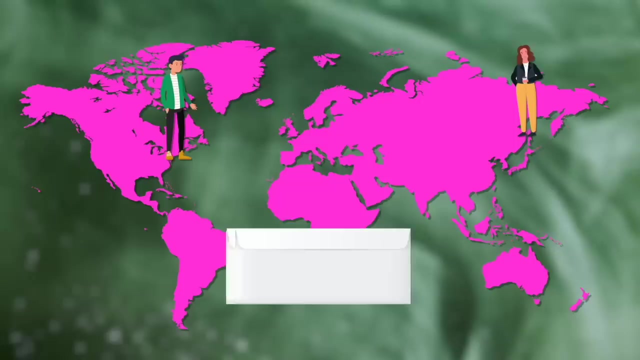 happen. There's no action at a distance, no portals. However, our descriptions of reality are not always local. Suppose I take two sheets of paper and write the number plus one on one and minus one on the other. I put them in two identical envelopes, Then I send one to Ellis in Tokyo and one 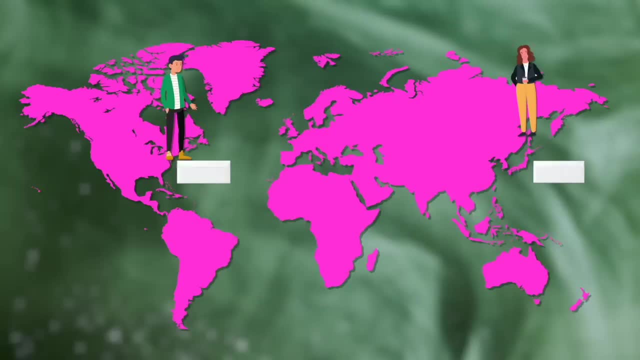 to Bob in New York, who is still waiting for Air France to deliver his bag. Ellis and Bob both know what I did, but not what's in their envelope. Either the plus one went to Bob and the minus one to Ellis, or the other way around. It's a 50-50 chance, But the 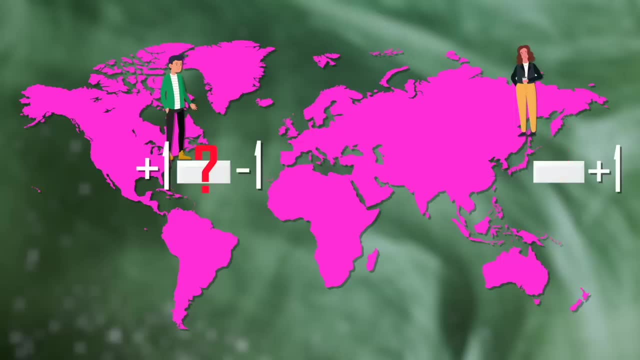 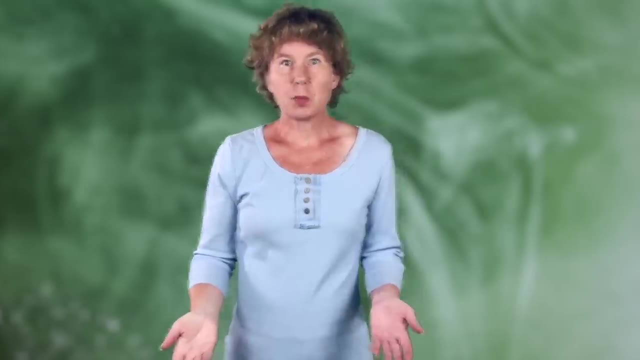 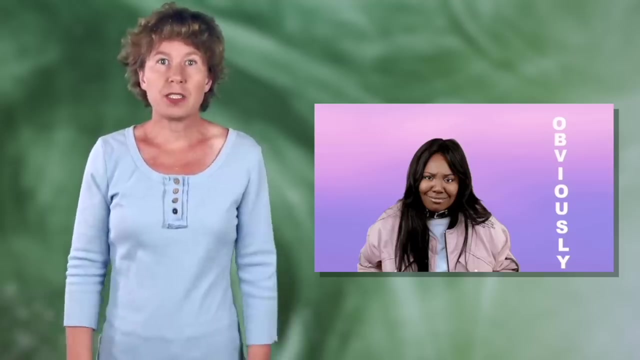 moment Ellis opens her envelope and finds plus one. she knows that somewhere in New York there's an envelope with the number minus one. You probably didn't find this particularly remarkable. Well, what did you expect? clicking on a video about locality? Only so much I can do to spice it up. 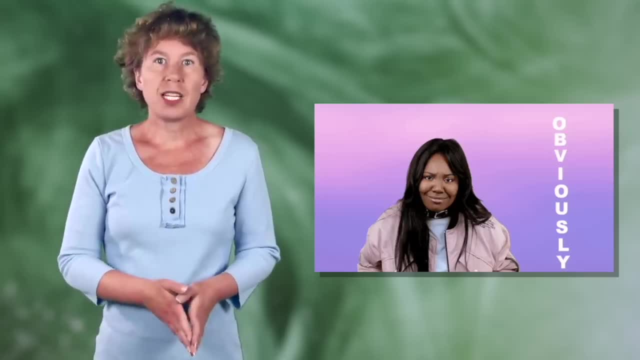 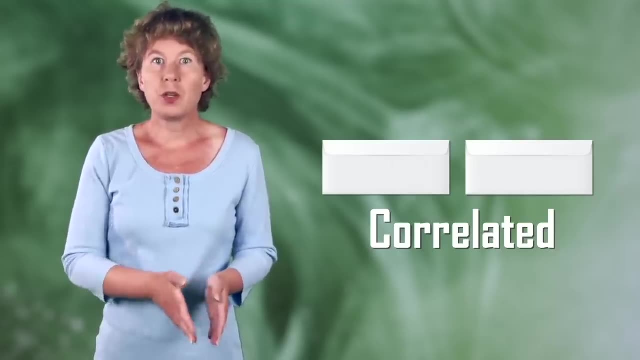 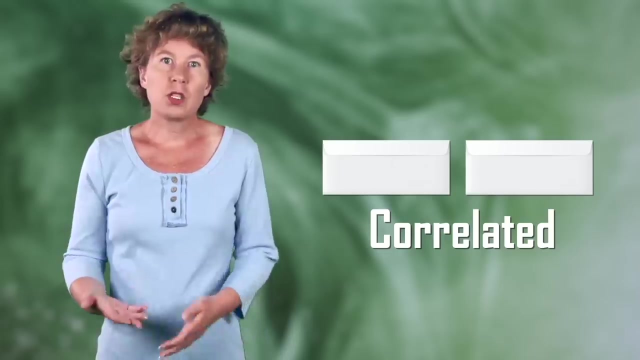 Remarkable or not, this simple example will be useful later. Thing is, these numbers in these envelopes are correlated. You don't know what either is, but if you know one, the other one is not random anymore And this correlation can stretch over a distance If you learn what one number in this correlated. 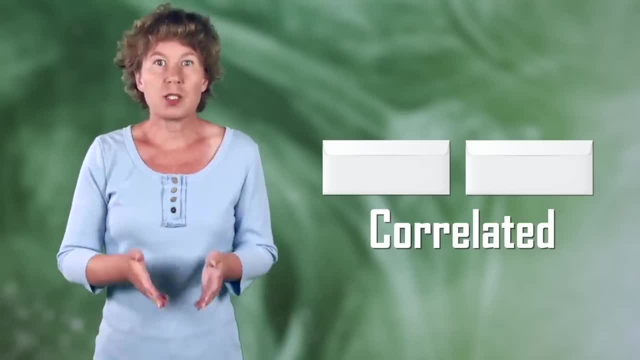 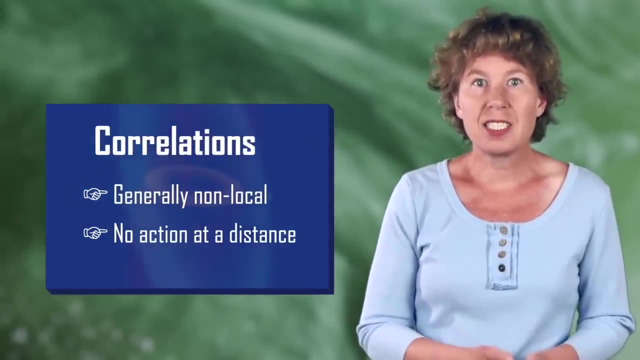 pair is you learn something about the other number elsewhere instantaneously. You could call that a kind of nonlocality, but it's not an action at a distance, It's distance. the only action that happens is an update of knowledge about something elsewhere. 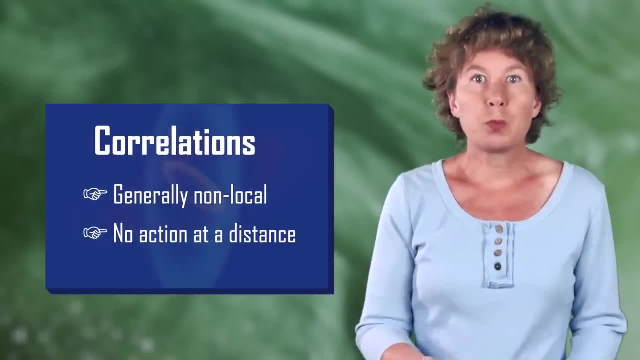 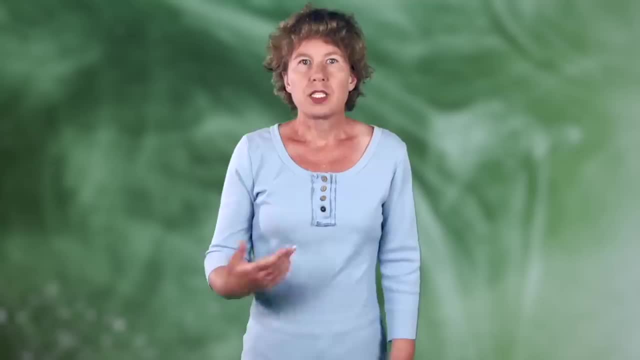 The action itself is completely local. It happens in Bob's brain or Alice's, unless maybe they've become so bored by my number games. there isn't anything left of their brains. So the lesson of the first part is there are two types of non-locality. 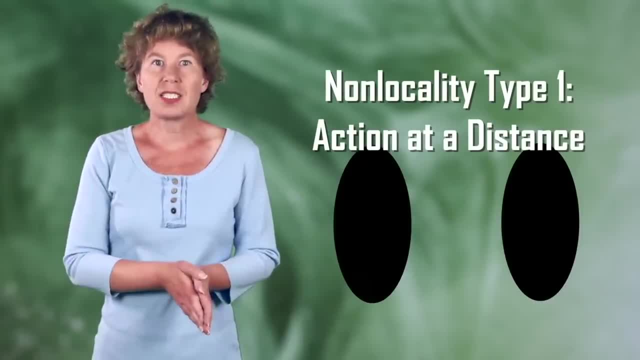 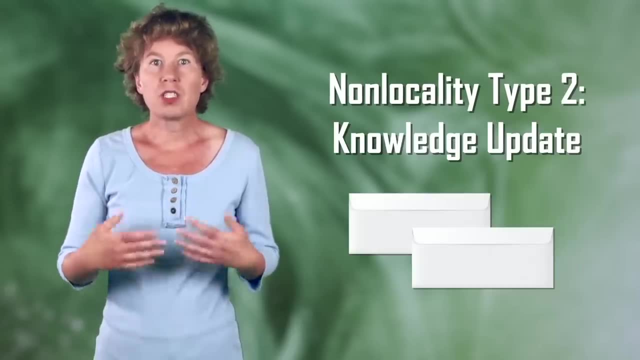 The one is a physical non-locality, an action at a distance, which is like something going through a portal. The other is a non-local correlation that allows us to acquire knowledge about what happens elsewhere, But in this case the only physical changes are local. 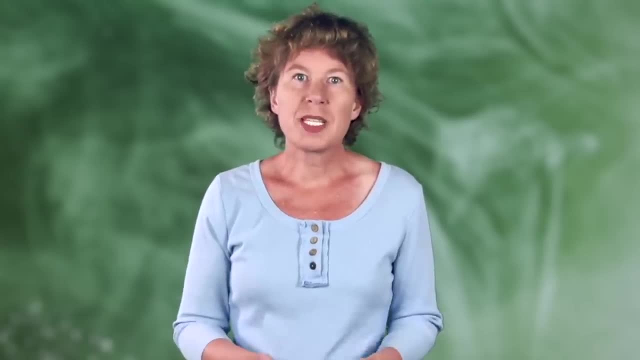 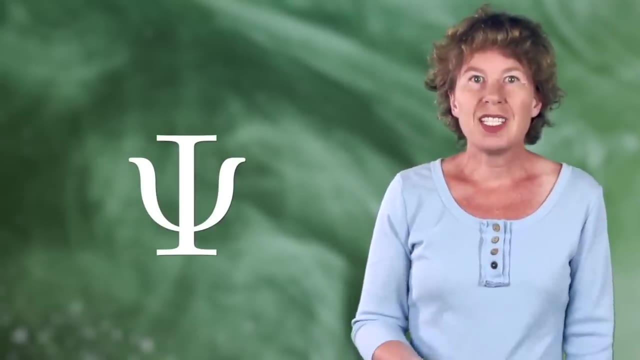 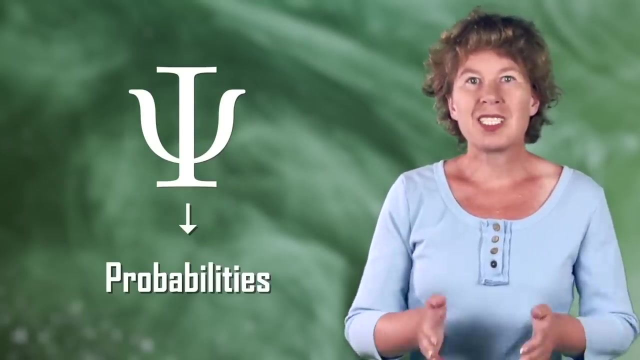 Let's then talk about quantum mechanics. In quantum mechanics, everything is described by a wave function, usually denoted with the Greek letter psi. The wave function is a device that we use to calculate the probability of getting a particular measurement outcome, But it doesn't predict the outcome. with science, 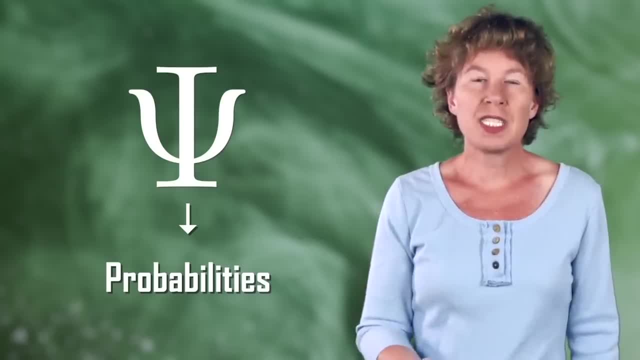 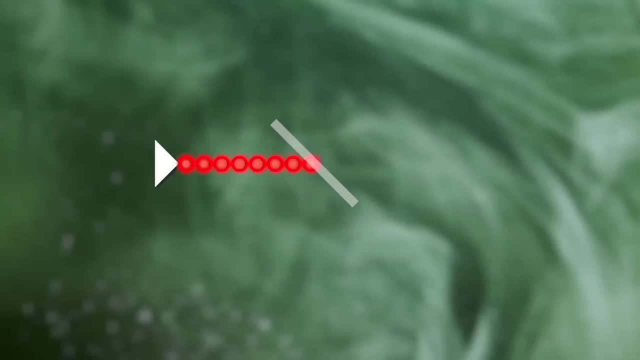 We say that quantum mechanics is not deterministic. Imagine, for example, you have a single quantum of light, a photon, and you send it through a semi-transparent plate. If you still have the space-time diagram in your head, please take it out and put it aside. 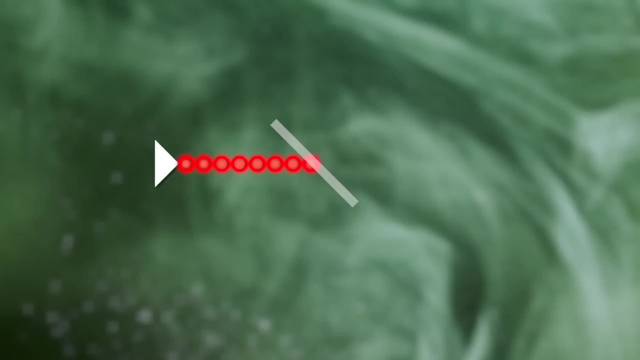 for now. This illustration just shows two dimensions of space. think tabletop. The photon has a 50% probability of going through the plate and a 50% probability of being reflected. So long as we don't observe the photon, its wave function changes locally from one 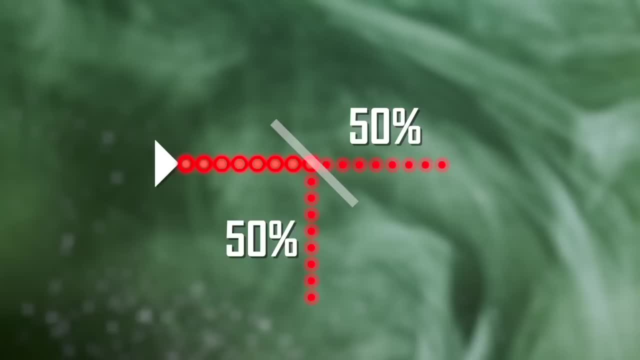 place to the next by spreading into these two directions. But once we make a measurement, we know where the photon went. Then the probability jumps to 100% on the one side where you've measured it and drops to 0% on the other side. 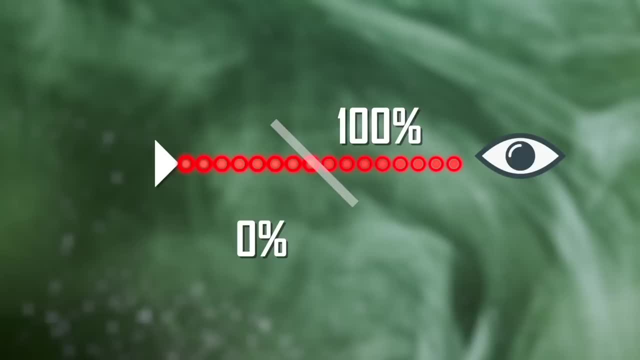 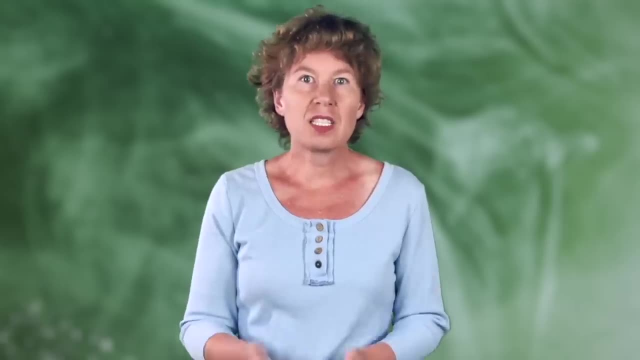 This is like when Alice opens her envelope and sees the number plus one. Now she knows that the probability of going through the plate is 0. The probability that Bob had plus one is 0. And, like Alice, adjusts her probability for Bob when she opens the envelope once we measure. 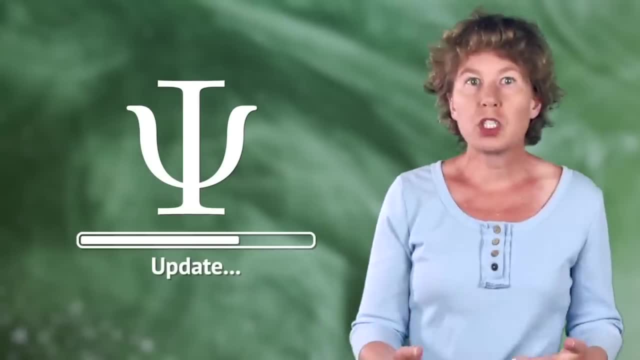 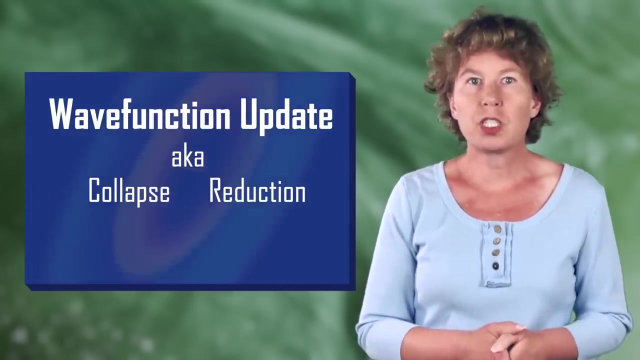 the photon on one side, we have to update the wave function to reflect this change in probability on the other side. Why? Because otherwise it doesn't agree with our observations. This update is also sometimes referred to as the collapse or reduction of the wave function. 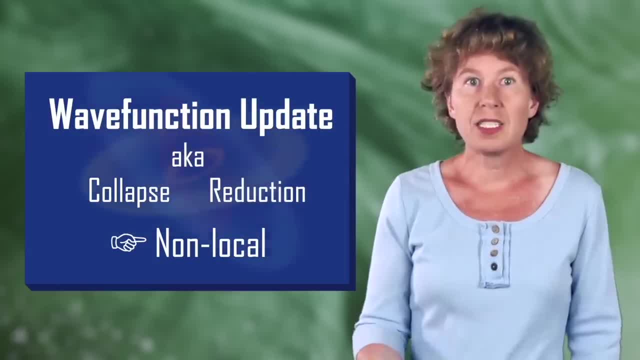 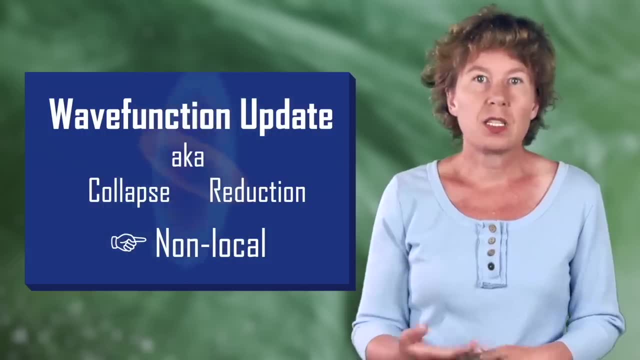 and it's non-local. You make a measurement in one place, Then you have the wave function: It's in one place and the wave function changes elsewhere. So quantum mechanics is non-local in some sense. The question is in which sense. 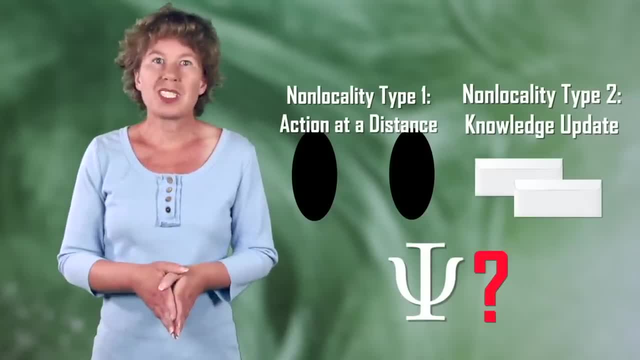 As we saw previously, just because you gain knowledge about something that happened elsewhere doesn't mean there was a non-local action. Maybe the wave function just describes knowledge rather than being real itself. Maybe the photon really went one way or the other, you just didn't know it. and the measurement? 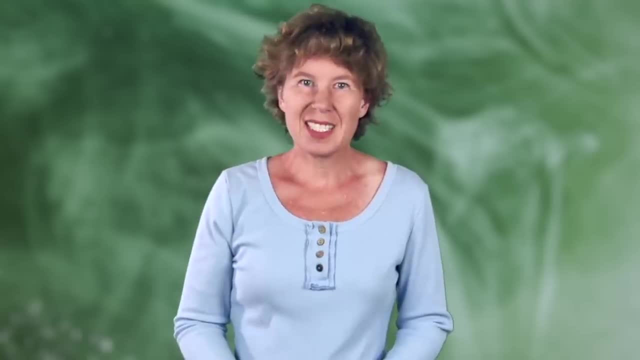 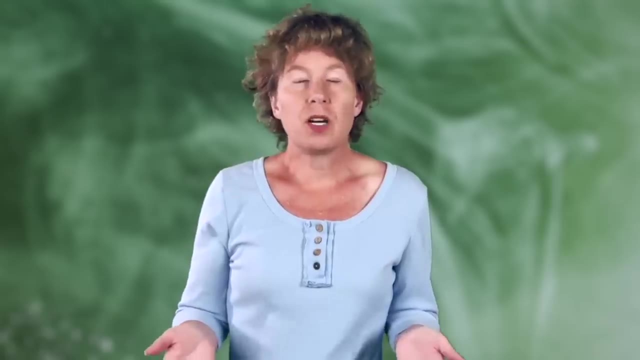 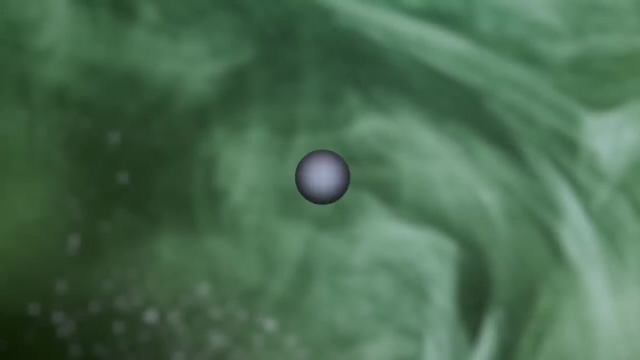 revealed its real state. Being a wave function isn't easy. Not only do people reduce and collapse you, they also then argue that it doesn't matter because you aren't real. The quantum mechanical version of the envelope example goes like this: Imagine you have a particle with spin zero that decays into two particles that can each. either have spin value plus or minus one. One flies to the left, the other one to the right. The total spin is conserved in the decay. So you know that either the particle going left has spin value plus one and the one going right has minus one, or the other way round. 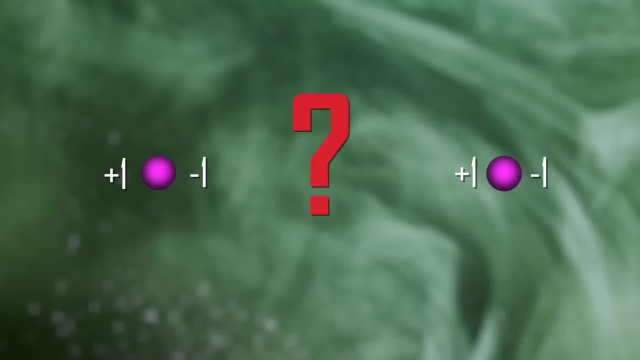 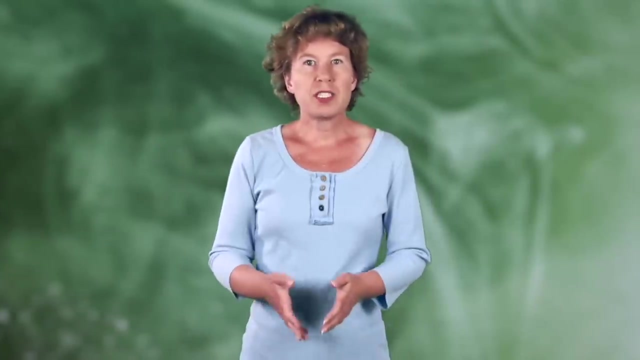 But you don't know which has which spin. These two particles are entangled. Entanglement is a correlation, like the correlation between the numbers in the envelopes, And like the correlation between the envelopes it can stretch over a distance. The difference between the two cases is that if you think that quantum mechanics is real, 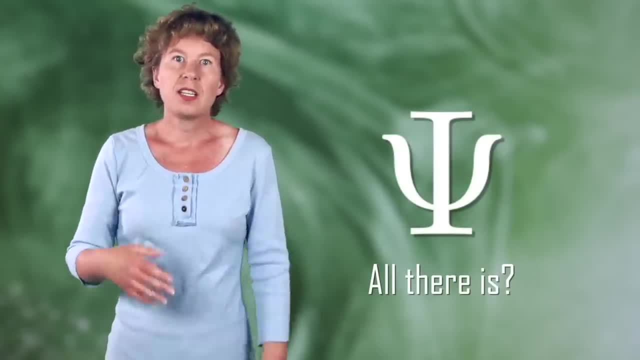 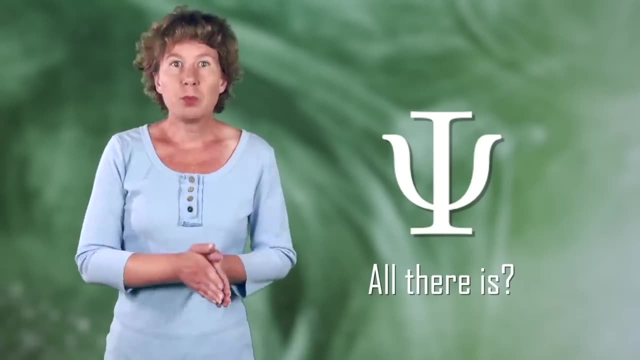 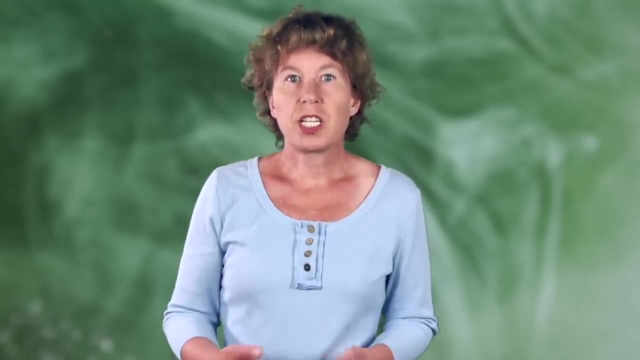 that quantum mechanics describes all there is. then, before you make a measurement, the particles really are in both states at once, and then the update is really physically non-local. The idea that this update is physically real is what Einstein called a spooky action at. 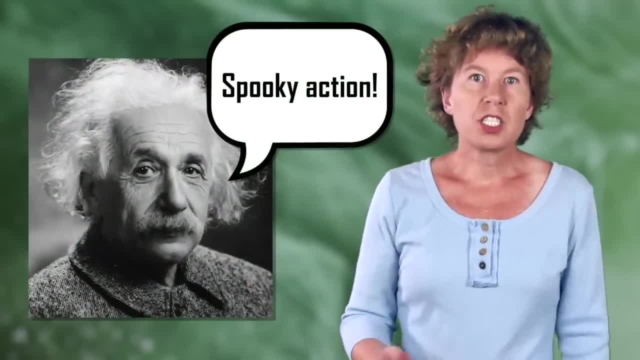 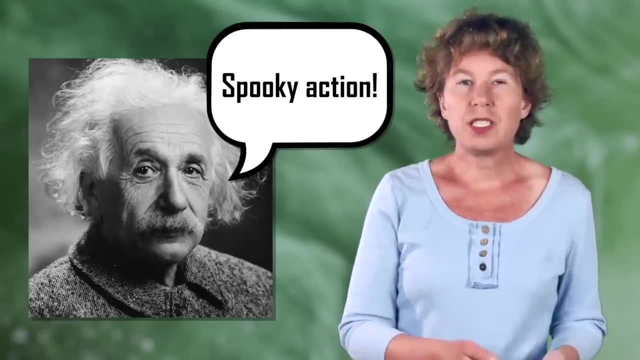 a distance. He thought that can't be right. Einstein believed that the real process must be local and that the update just revealed it. And that's exactly what he said. He said that the wave function is all there is and the collapse is really non-local. 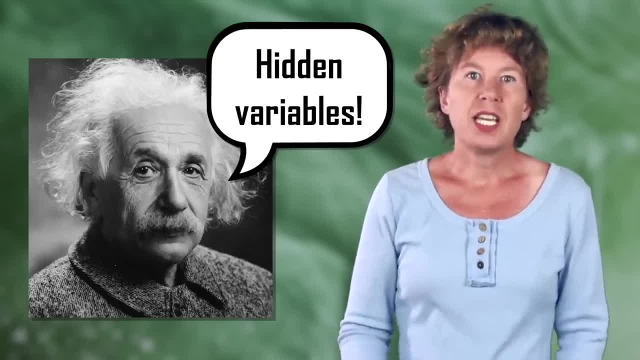 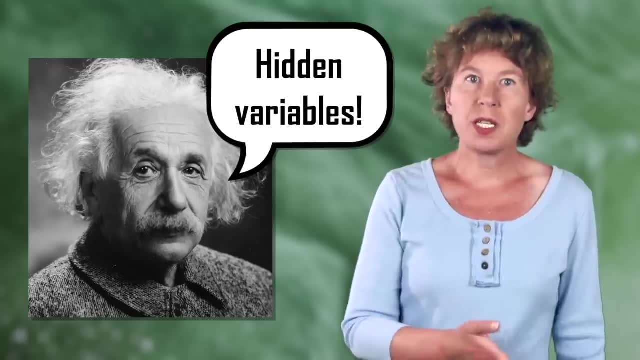 That's something you reveal in a measurement- is usually called the hidden variable. It could be, for example, the value of the spin that the particle really had before you did the measurement and found out what it is. Bohr held against that. 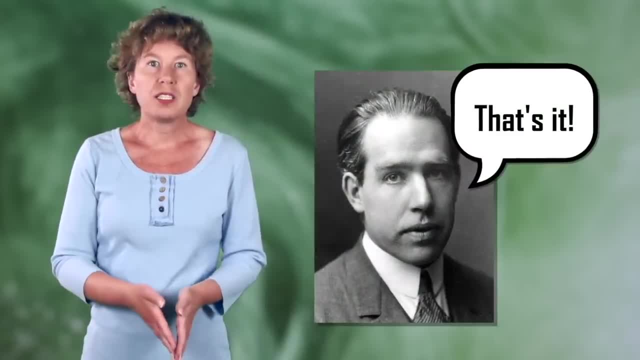 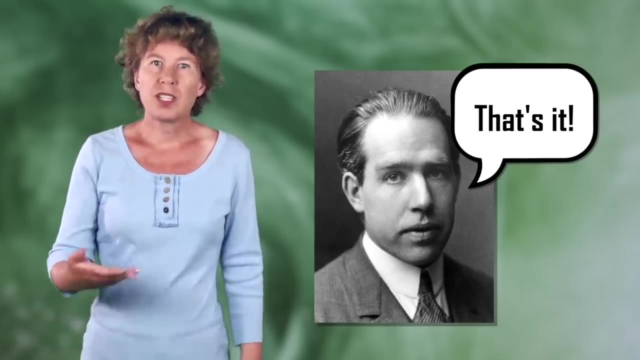 He said, there are no hidden variables and no underlying information that you can reveal. The wave function is all there is, and the collapse is really non-local. Bohr seems to have liked quantum mechanics Because he thought that its indeterminism makes place for free will, though that's. 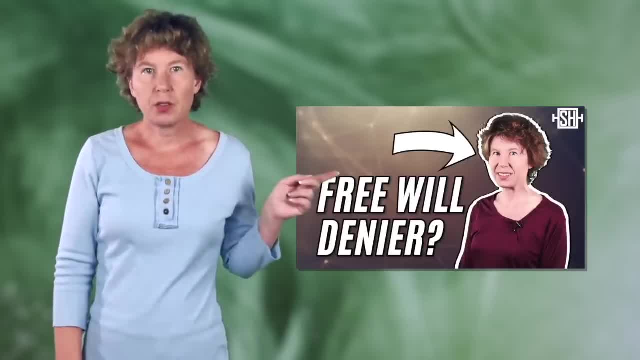 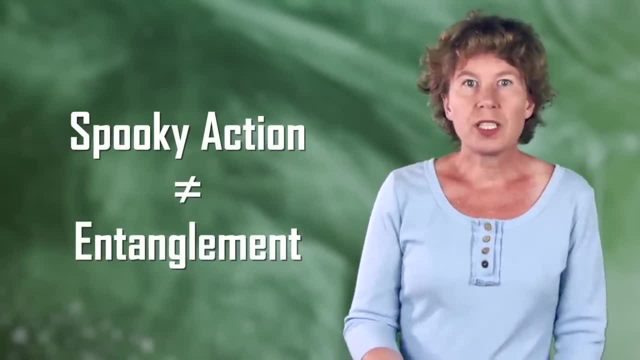 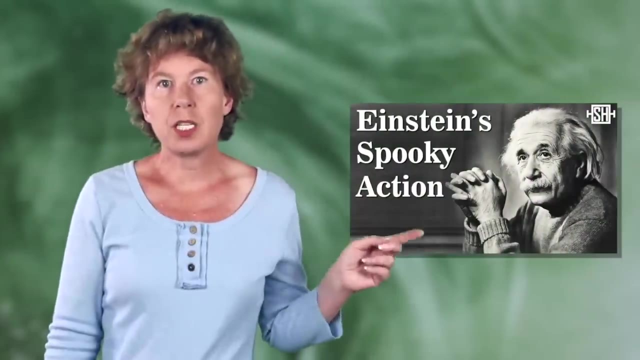 rather questionable. We just talked about that a few weeks ago. Einstein did not use the phrase spooky action at a distance to refer to entanglement. To begin with, the example in which he coined the phrase didn't use entangled particles. I went through the history in a previous video. 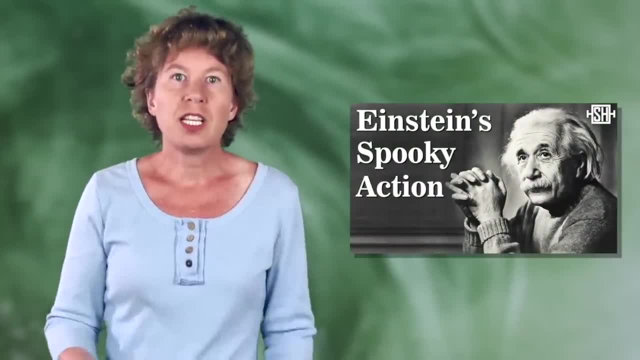 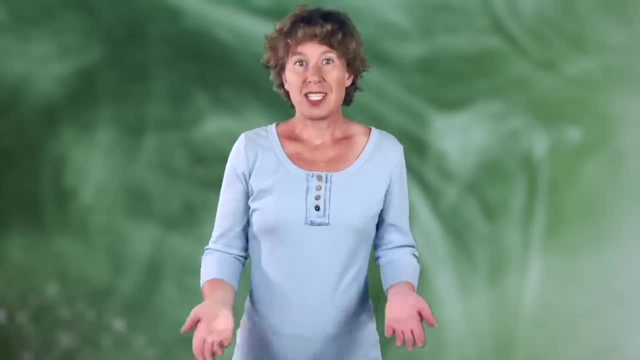 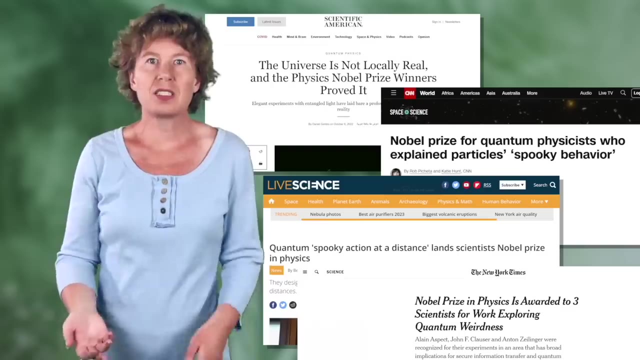 But, more importantly, entanglement has no action. It's just a correlation, A correlation that stretches over a distance, like the correlation between the envelopes. When I read the headlines about last year's Nobel Prize, I got the impression that some science writers believe entangled particles are somehow mysteriously linked to each other. 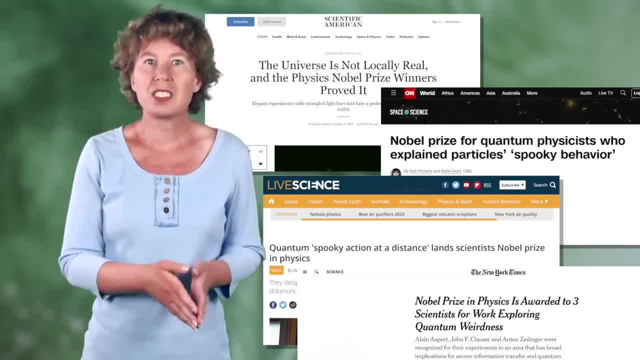 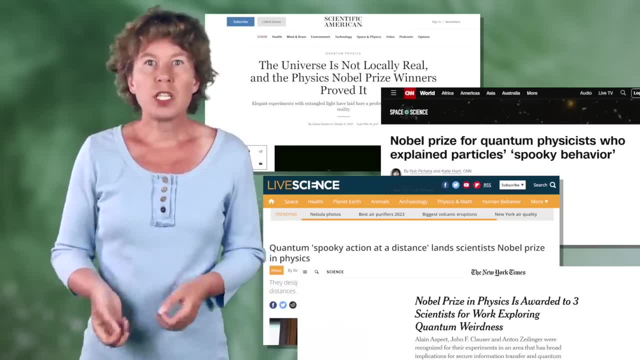 They seem to think that if you do something to one particle in an entangled pair, then that'll immediately affect the other one. But this isn't so. It's only when you measure one particle, Then you have to update the wavefunction of both. 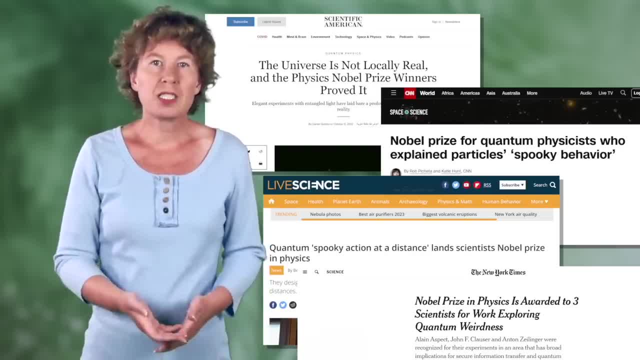 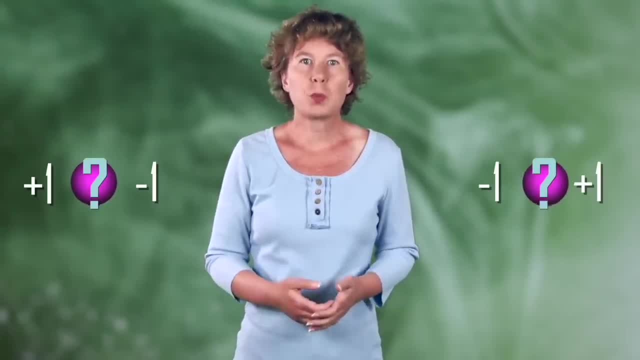 So long as you don't measure them, doing something to one particle won't affect the other one. You could, for example, flip the spin of one of the particles in an entangled pair so that one becomes minus one, and the other way round. 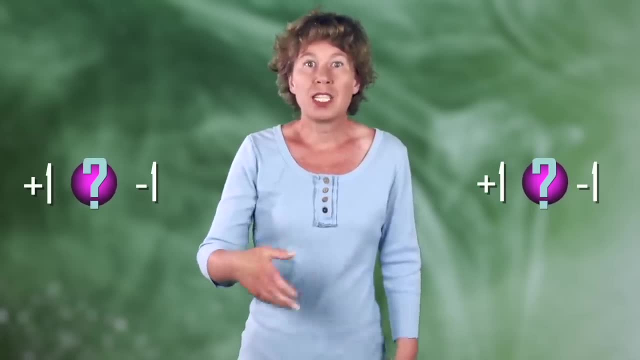 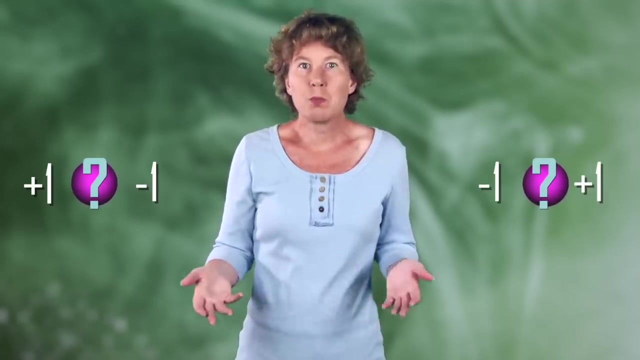 You can do that without measuring the spin, Like you can do this in reality in the laboratory, not just with mathematics. If you flip the spin of one particle without measuring it, it This'll not do anything to the particle it's entangled with. It's not as weird as they made you. 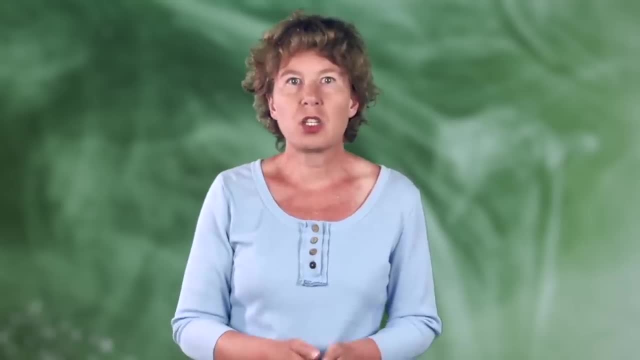 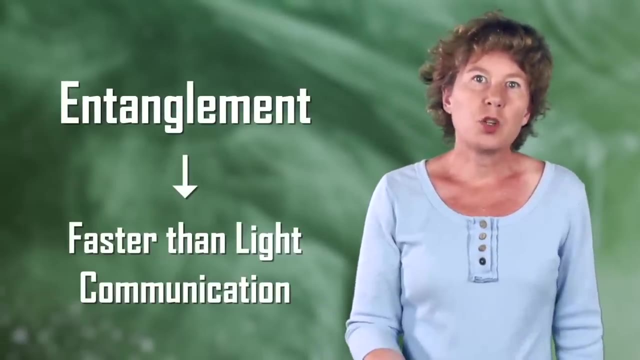 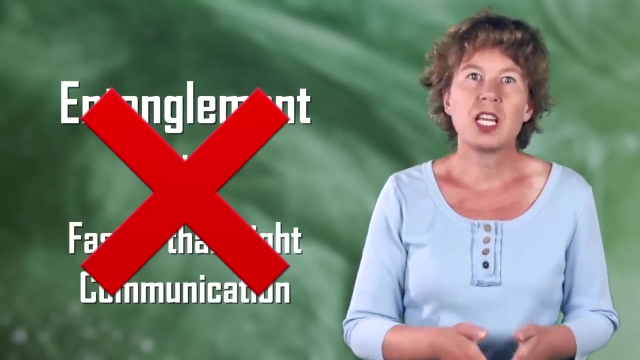 believe it is, is it Okay? so entanglement is just a correlation over long distances, But does it at least allow us to send signals faster than light? Unfortunately not. It doesn't work because you can't force the outcome of your measurement on one of the entangled particles to 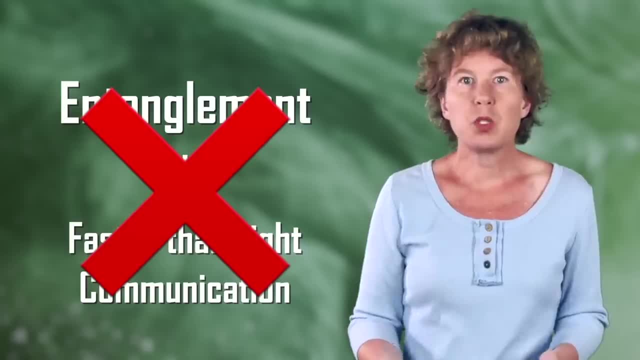 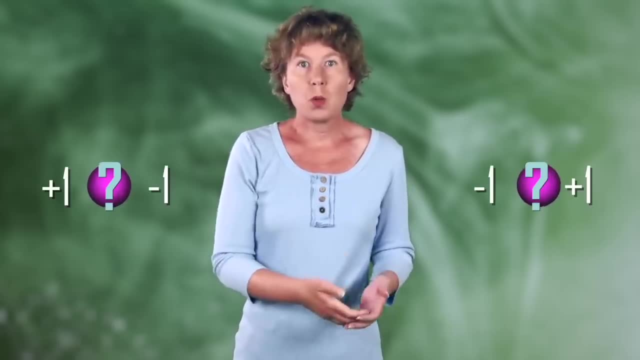 be a particular value. It'll just be randomly distributed according to the probability given by the wave function. This means that on the other end, they won't know whether you have made a measurement, any more than Bob knows whether Alice has opened her envelope. If quantum mechanics 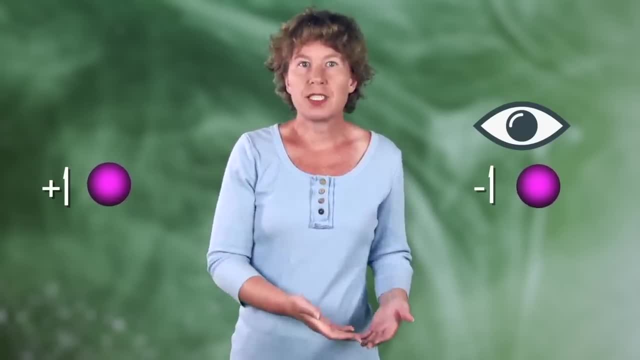 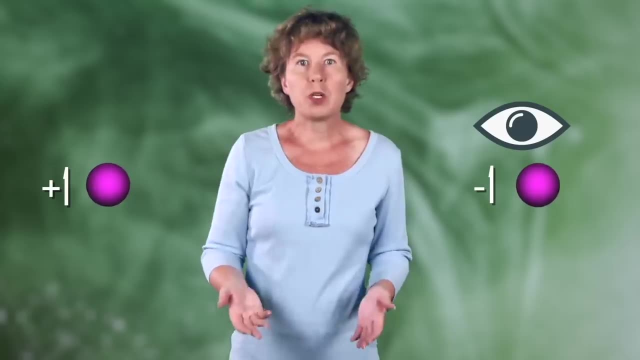 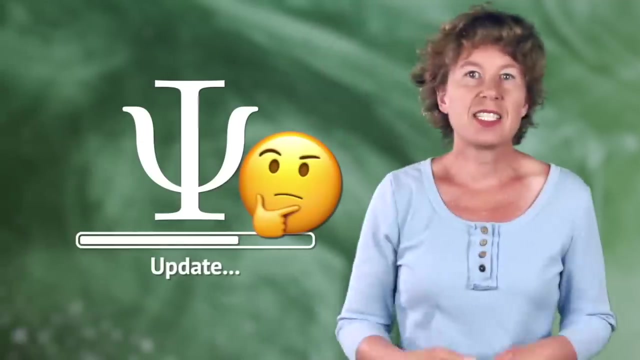 is correct, then no information can be sent faster than light. One can mathematically prove that this is the case, not just for this experiment, but for any possible experiment. It's called the no-signaling theorem, But because of this randomness of quantum mechanics it's also rather hard to predict the outcome of your measurement. You can't predict the outcome of the wave function. This means that on the other end, they won't know whether you have made a measurement, any more than Bob knows whether Alice has opened her envelope. It's also rather 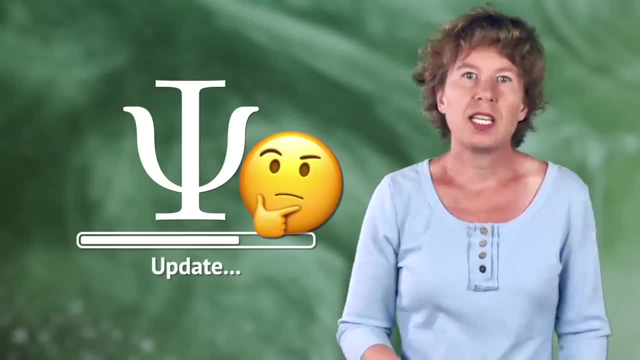 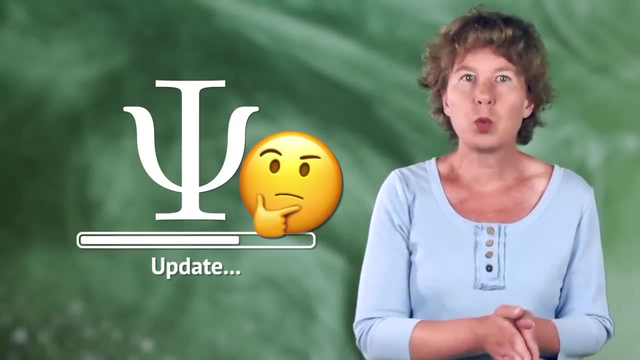 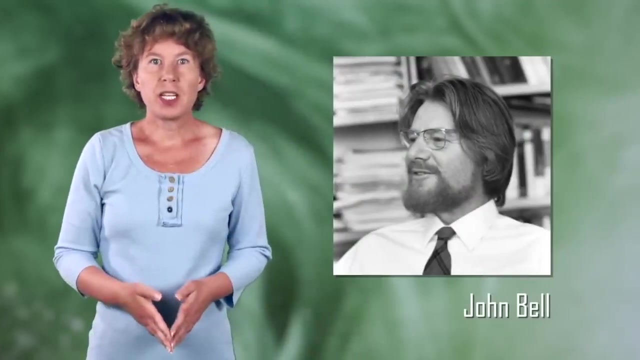 unclear, in which sense the collapse is even non-local. If making the measurement on one of the pair of entangled particles doesn't change the measurement outcome on the other one, then what is non-local in the first place? Enter John Bell. Bell tried to find a way to. 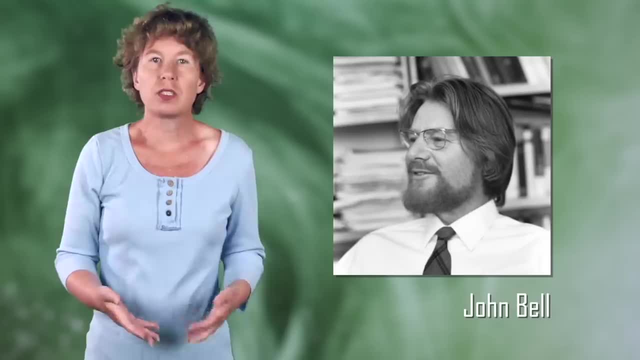 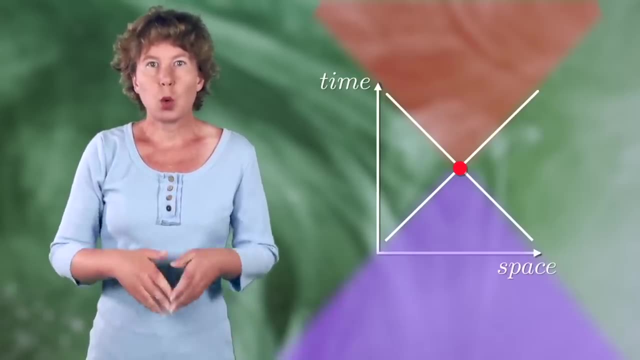 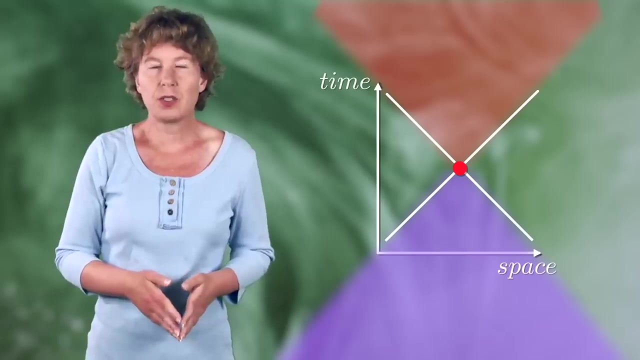 pin down what it means that quantum mechanics is non-local. Please put the space-time diagram back into your head, because we need it again. We've seen earlier that without faster-than-light travel, everything that an event might be influenced by has to be in the past light cone. 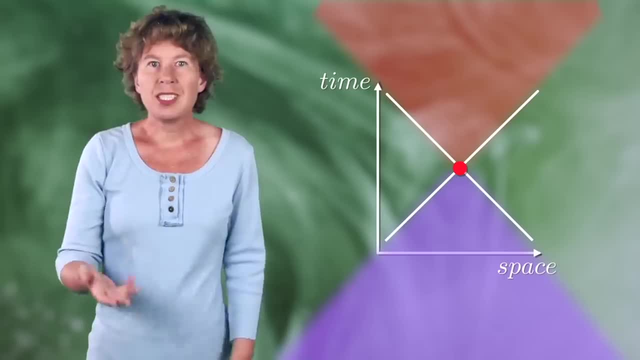 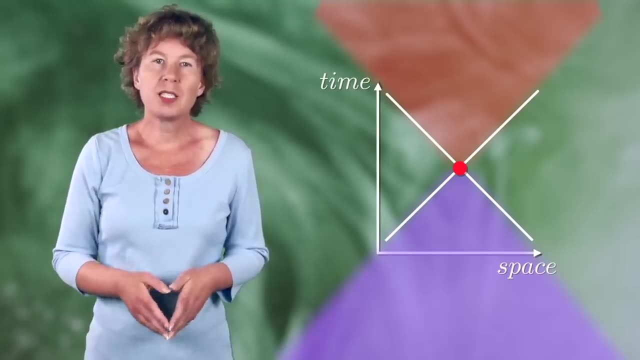 But if the theory is also local, then you don't need the entire inside of the light cone. This is because if you know what happens at one moment in time, you can calculate what happens later. If the theory is deterministic, you can calculate it. 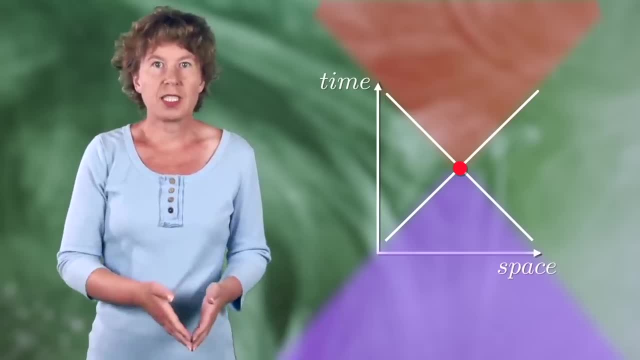 exactly If it's not deterministic. probabilistically, This means all you need is the information at one particular moment in time. for anyone's notion of time In one dimension, that moment is a line going through the inside of the past light cone. In three dimensions, 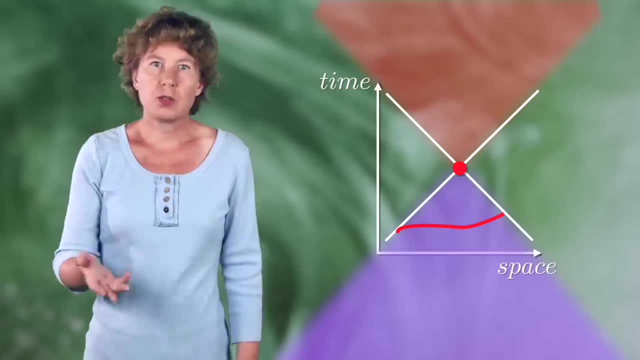 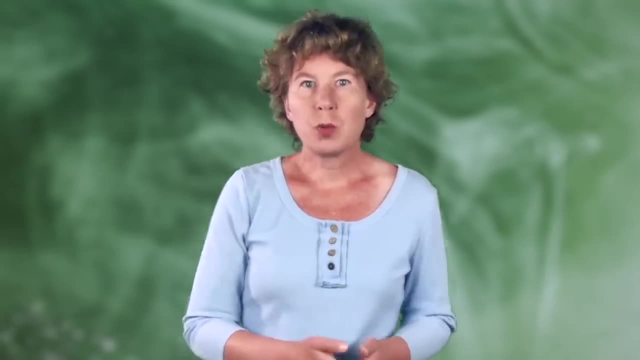 it's what's called a space-like hyper surface. just so you don't go away disappointed about the lack of incomprehensible terminology. The point is that the information at one moment in the past- light cone of the event- is all you need to calculate what happens at the event. If the theory is local, the idea remains to be hoy for the next generation, Unless there's a wishing for a good future. only then will we be immune to a future leaning in the ценza. Хорошо Become. 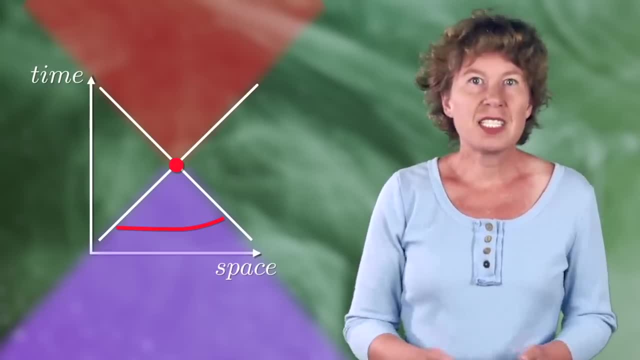 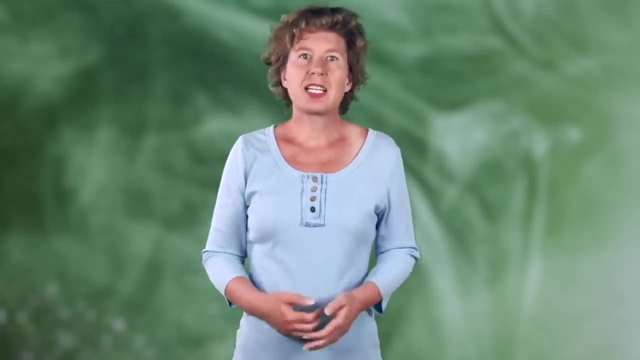 ofman, If the theory isn't local, then that doesn't work, because information could jump into your light cone later. Bell's insight was now that you can use this to decide whether the theory is local And it works, even if the theory has a random element. 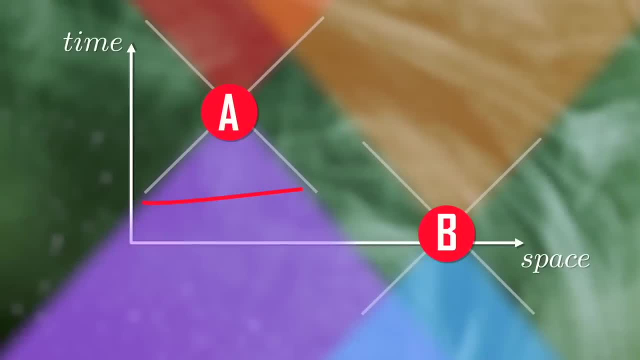 Suppose you have all available information on this slice here And you use that to make your best prediction for what happened here, Then the theory is local. if information from over here doesn't tell you anything new about what happened at A Bell called this property, local causality. 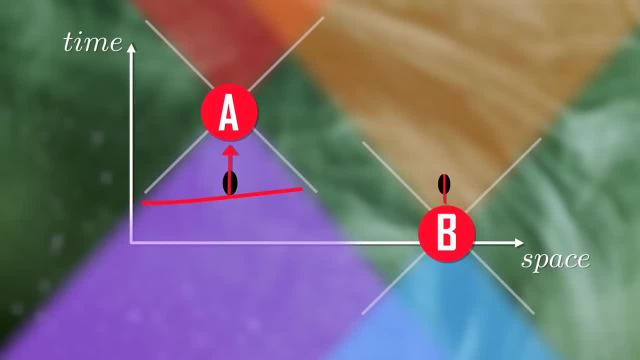 If, on the other hand, the theory is not locally causal, then information can jump into the light cone after your slice, And that can tell you something about what happens at that event. Quantum mechanics is not locally causal. Think back of the earlier example with the entangled power. 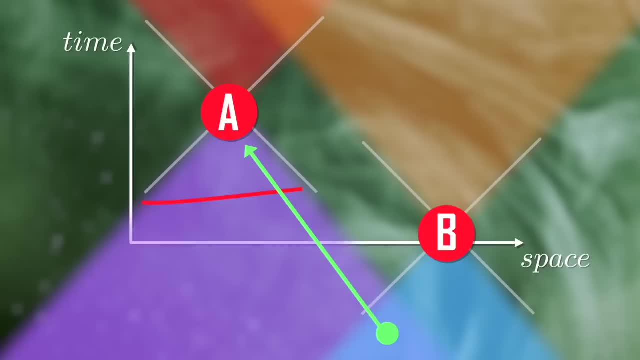 Particles, Let's say they are created here. One goes left, one goes right. In the spacetime diagram this means they go diagonally, no less than a 45 degree angle. You make two measurements here and here let's call them A and B. We want to know what happens. 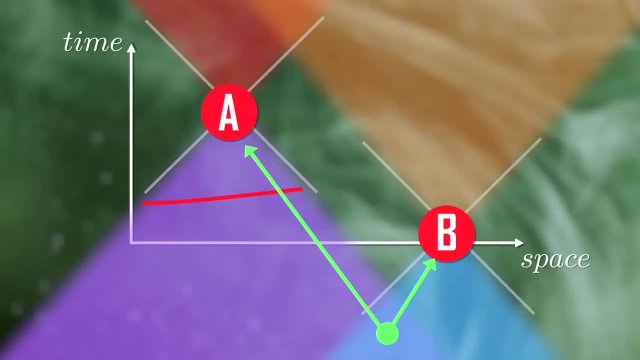 at measurement A. All the information you could have about it is down here in the wave function. This wave function, as we've seen earlier, does not allow you to predict the measurement outcome at A, Just the particle, The probability of a measurement outcome. 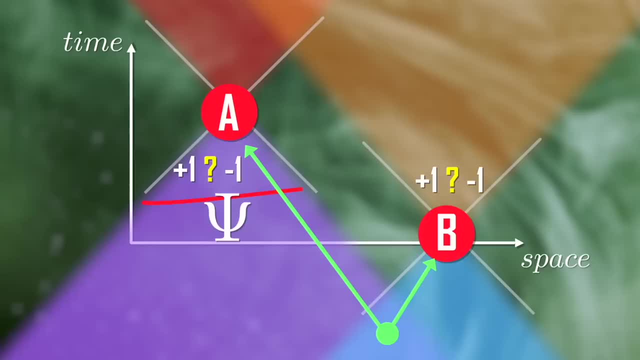 It's either spin minus one or plus one, with 50% probability each. Here's the thing: If you make a measurement over here at B and you find it's plus one, then you know the spin at A is minus one. So what happens at B does add information to the inside of the past light cone and quantum. 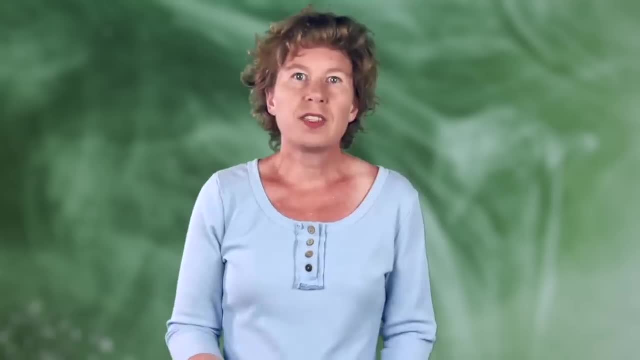 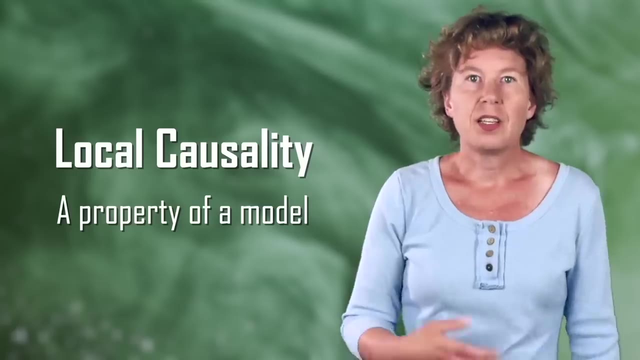 mechanics is not locally causal. The important thing is now that local causality is a property. So what happens at B does add information to the inside of the past light cone and quantum mechanics is not locally causal, In this case a property of quantum mechanics. 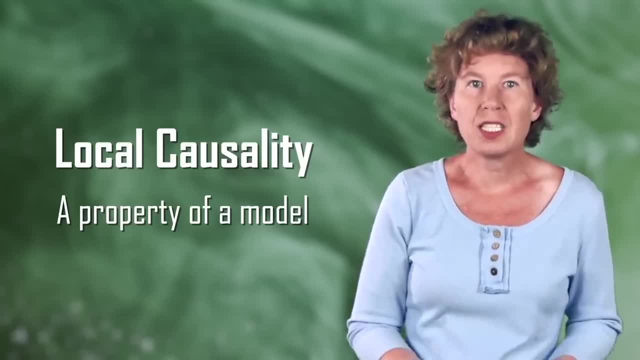 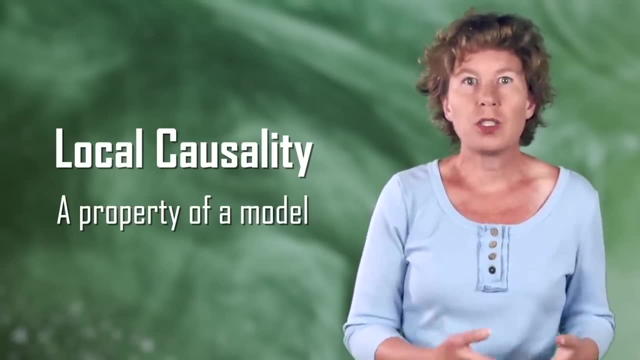 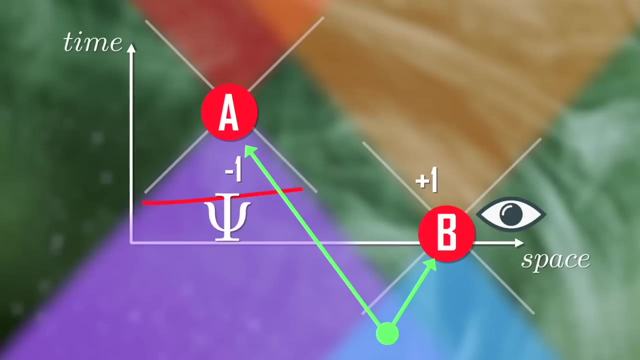 The relevant question is whether it's also a property of reality. If quantum mechanics was all there is, then that'd be the case. The wave function would be how the world really works, And it would have a spooky action at a distance. But if quantum mechanics was not all there is, then the wave function down here was not. 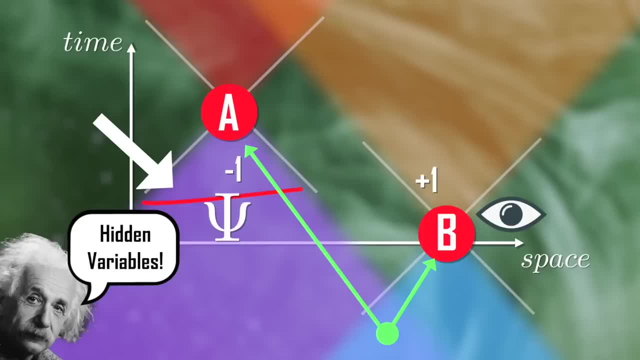 the entire information. That'd be a hidden fact, hidden variable there, from which the outcome followed. And if you had had the entire information, then adding the measurement outcome from B would not provide any further information. Quantum mechanics would still not be locally causal, but reality would be. 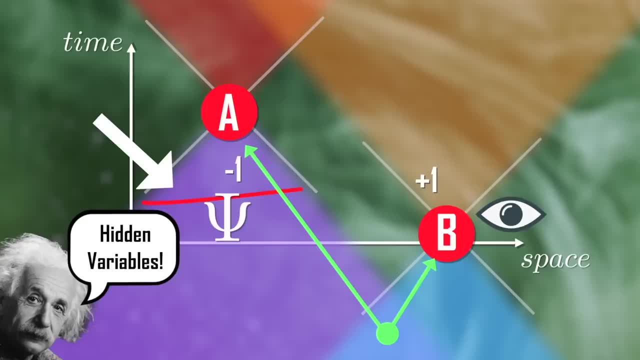 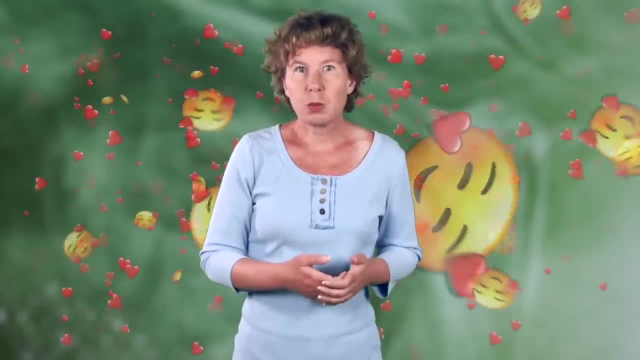 So which one's right? That's what Jean Bell was trying to figure out. Wow, you're still with me. that's lovely. I really appreciate the company. Let's look again at that semi-transparent plate, because it can teach us something very important. 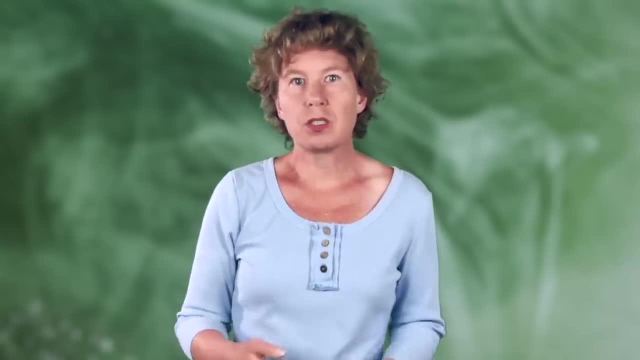 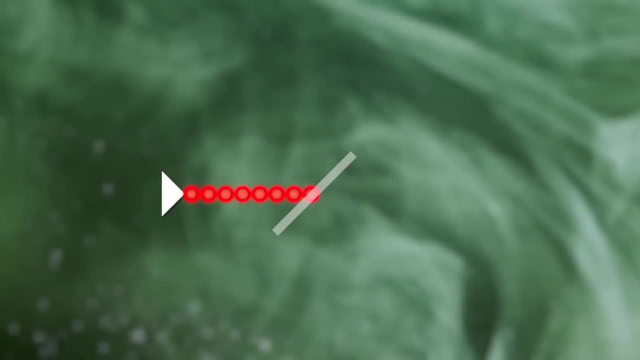 We'll now try to build a simple hidden variables model that explains what happens at that semi-transparent plate, also called a beam splitter. We want to do this with hidden variables and we want to do it locally, so no action at a distance. 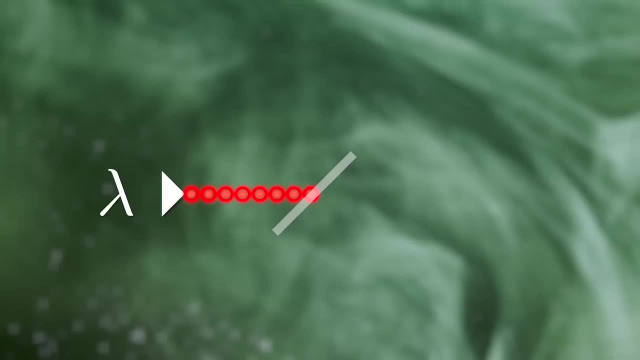 The hidden variables are usually called lambda. So we'll say if lambda is 1,, then the photon goes that way, if lambda is 3,, then it goes the other way. Why 3 and not 2?? Because I know what's coming next and you don't. 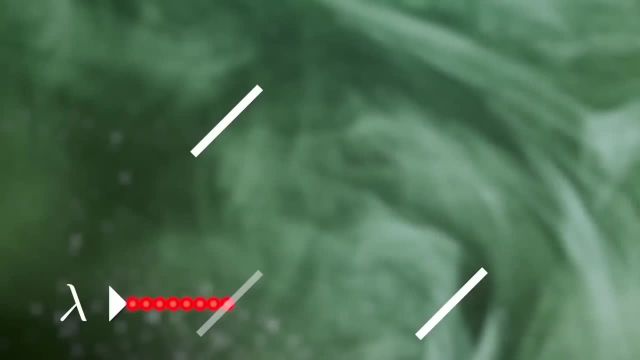 Now we put two mirrors here and here so that the photons don't run off our screen, and another two semi-transparent plates there. Okay, so now we have four different paths, each with 25% probability. We'll give those the numbers 1,, 2,, 3,, 4.. 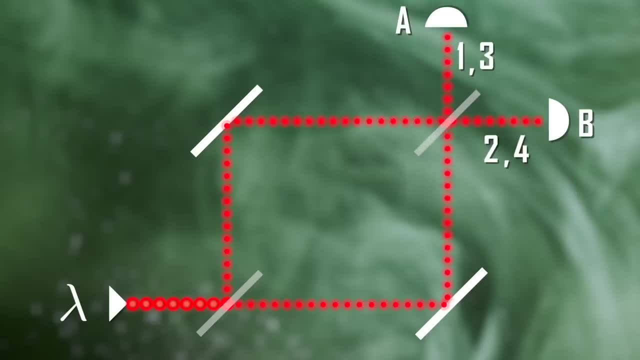 And now we'll combine these two paths by directing both towards the same beam splitter. If our hidden variable explanation was correct, then we should get half of the photons here in detector A and half here in detector B. But this isn't what happens. 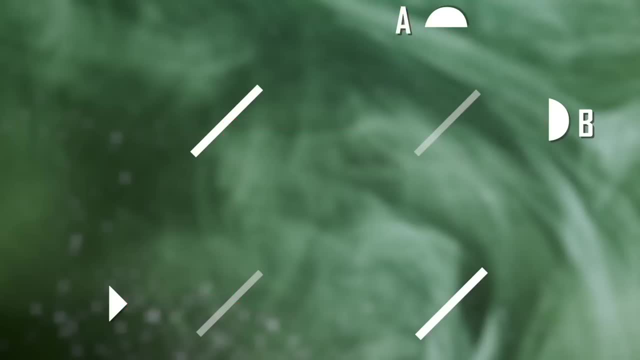 Indeed, you have probably noticed that this setup is what's called a Mach-Zehnder interferometer. If the paths are the same length, then the photon will always go to detector B. You can measure it and all. it's definitely real. 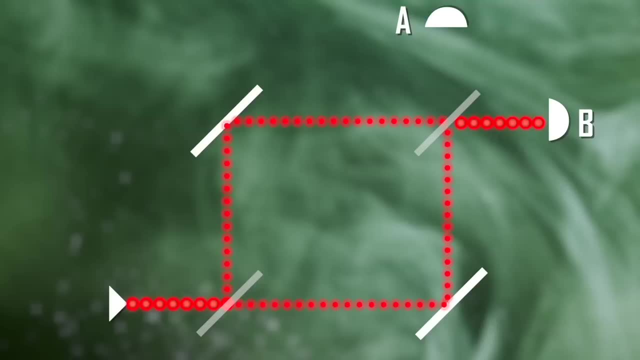 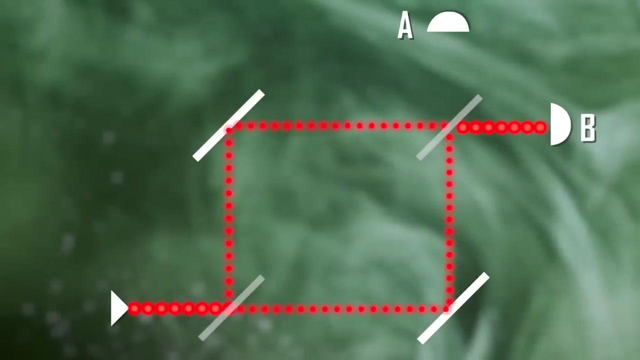 The interference in these detectors is exquisitely sensitive to the length of the paths, which is why one can use this type of interferometer to measure tiny deformations. This is how a gravitational wave interferometer works. But how does it work? Well, in quantum mechanics, the photon is described by a wave function. 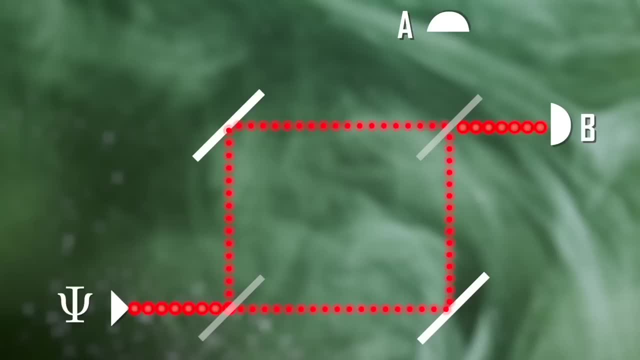 and waves can interfere with themselves either constructively or destructively. In quantum mechanics the photon goes over both paths and on this output the wave interferes destructively with itself. so no signal and all photons go the other way. But the price you have. 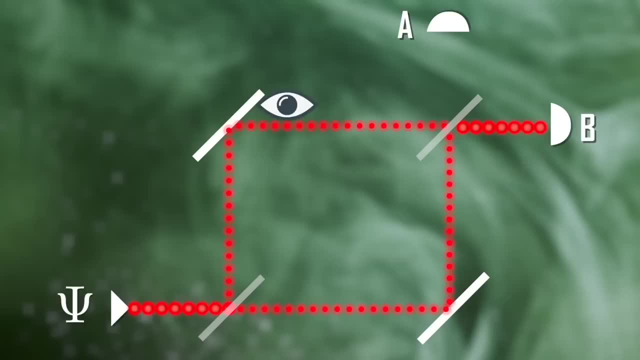 to pay for this is that if you measure which path the photon went, you need the non-local collapse. How can we use hidden variables to get this done locally? Well, no one's ever said that we can't have waves that go two paths in a local hidden variable. 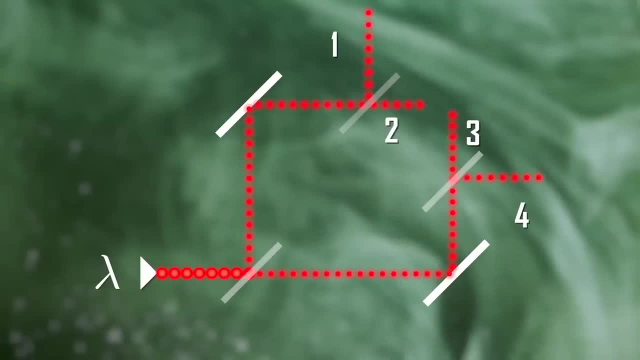 model. We can't have waves that go two paths in a local hidden variable model. All we need to do is say: if we measure which path the photon goes, then we use these variables- 1,, 2,, 3,, 4, and the photon behaves like a particle. 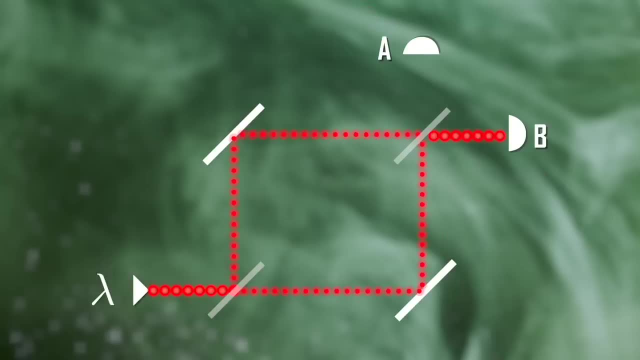 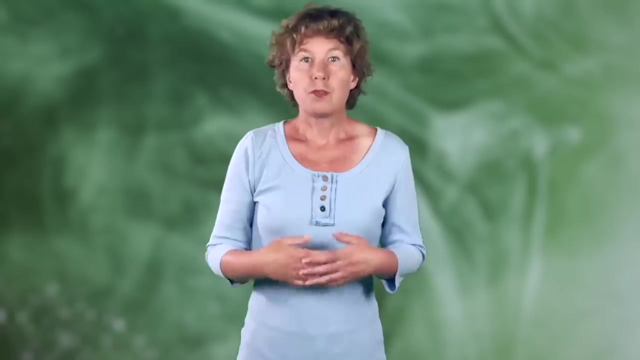 If we measure the interference between the paths, then that's hidden variable number 5, the photon behaves like a wave and goes only into detector B. problem solved. It's local because the photon goes on one continuous path into the detector where it's measured. For this to work, 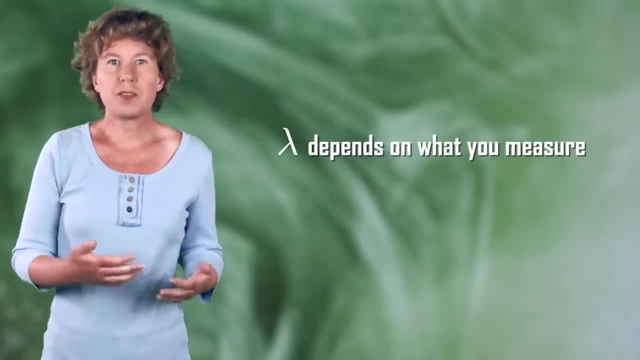 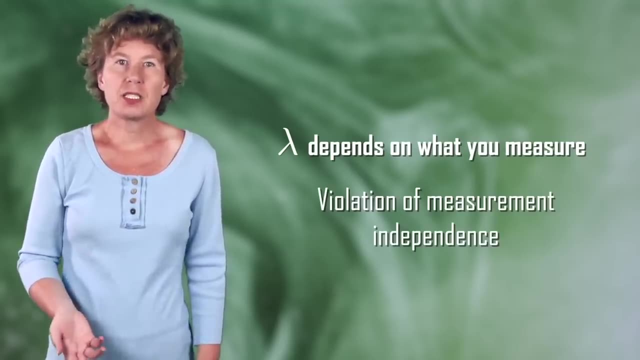 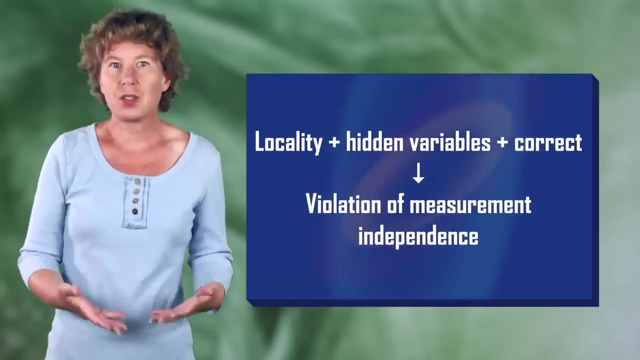 the value of the hidden variable that determines what the photon does must depend on what you measure. It's called a violation of measurement independence. So the lesson is: if we want a local hidden variable model that reproduces quantum mechanics correctly, then it needs to violate. 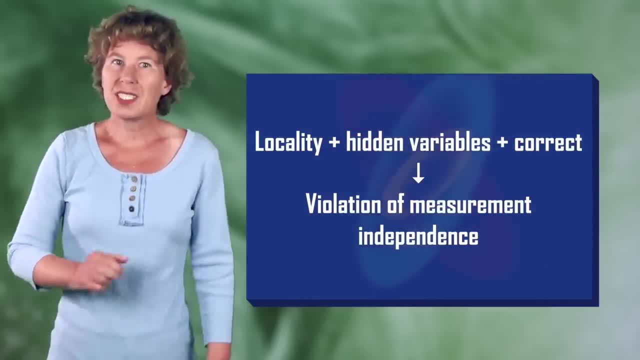 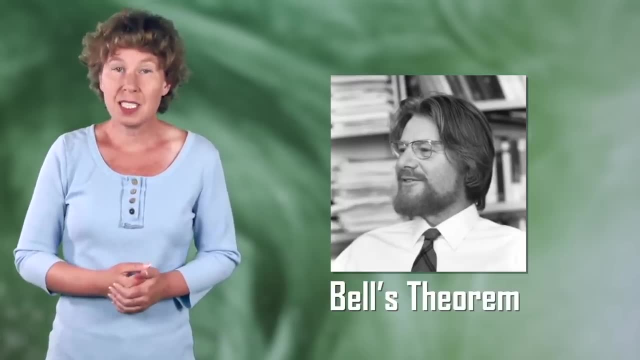 measurement independence. This finally brings us to Bell's theorem. I'm not going to explain Bell's theorem because you've already watched twenty videos about it and you're not going to understand it and it didn't help. I'll just tell you what it says. Bell's theorem says, if you want. 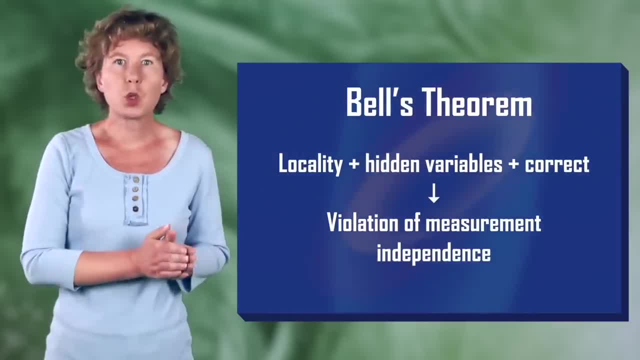 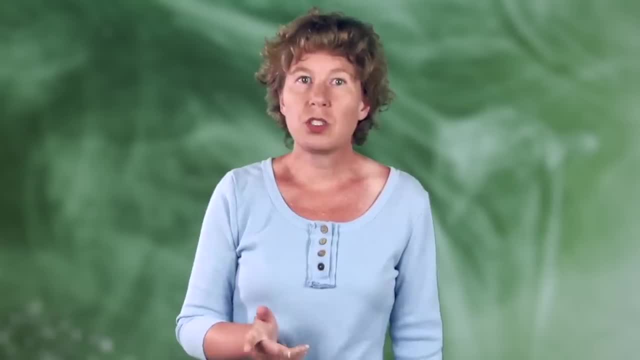 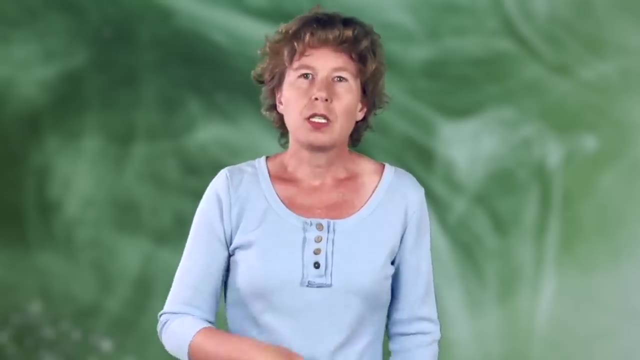 a local hidden variables model that reproduces quantum mechanics correctly, then it needs to violate measurement independence. Isn't that what we just concluded from this little example with the interferometer? Yes, Bell's theorem says the same thing. You see, what happened is that Bell? 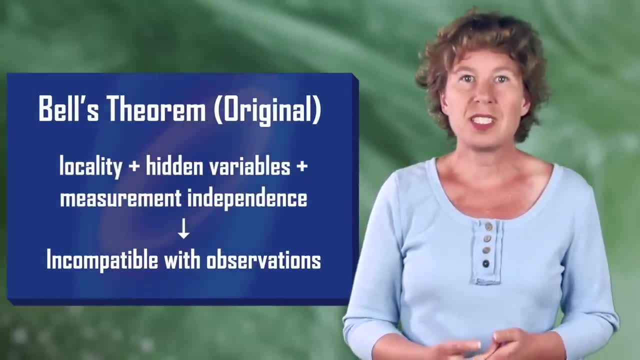 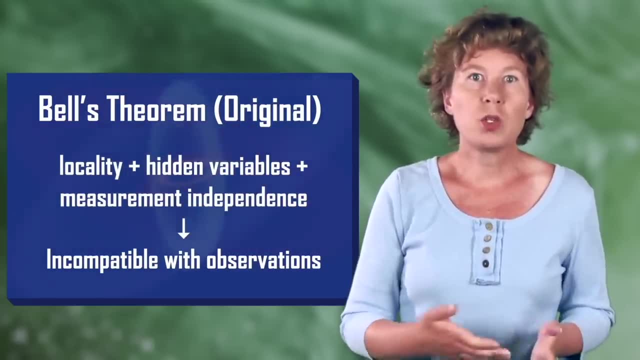 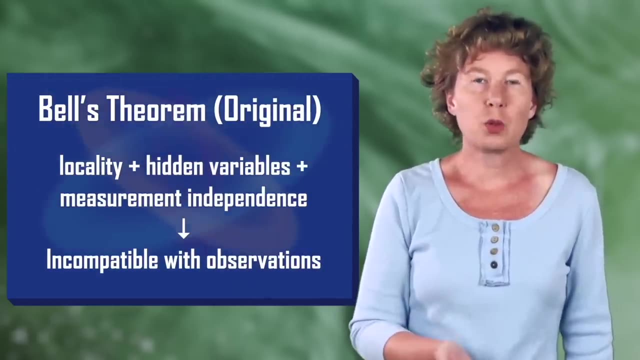 originally just assumed that measurement independence is a function of the quantum mechanics of the scale. He then proved that any local hidden variables theory which fulfills this assumption will obey an inequality for the correlations of certain measurement outcomes. It's now called Bell's inequality. Quantum mechanics can violate this inequality. 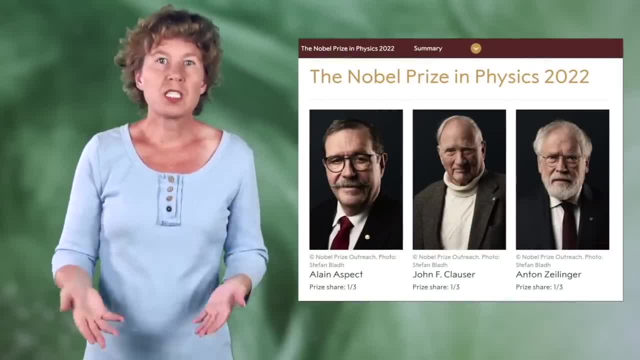 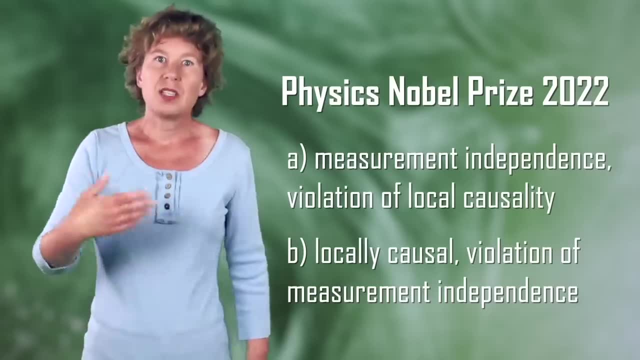 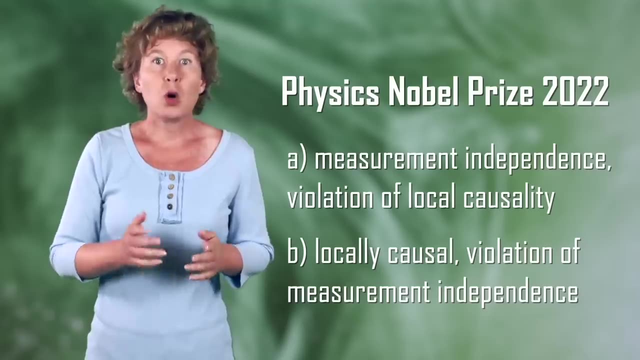 What the Nobel Prize was awarded for is experimentally demonstrating that these inequalities are indeed violated by observed measurement outcomes means that either reality respects measurement independence but is not locally causal, or it's locally causal and violates measurement independence. Just logically, it could be. 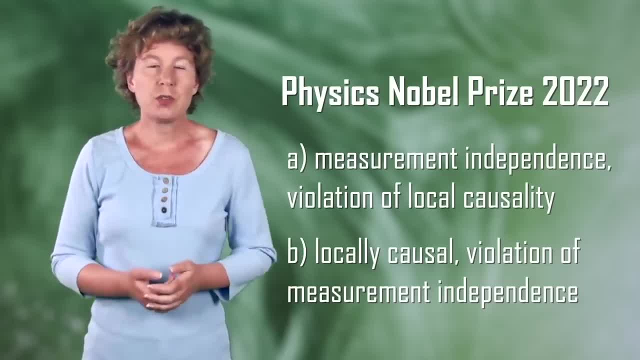 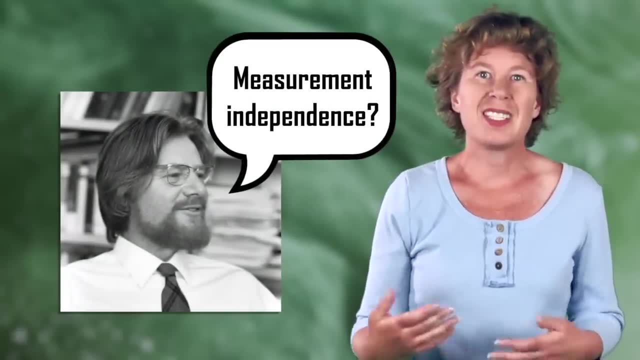 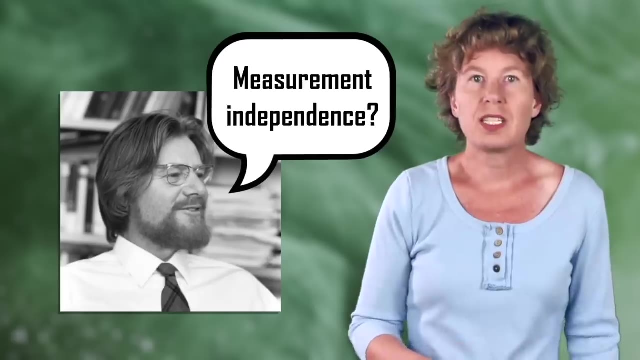 a combination of both, but I don't know why you'd want to do that, Since Bell had forgotten about this assumption of measurement independence. he mistakenly thought that demonstrating an experimental violation of his inequality would rule out all local hidden variables models and thereby show that spooky action at a distance is real. 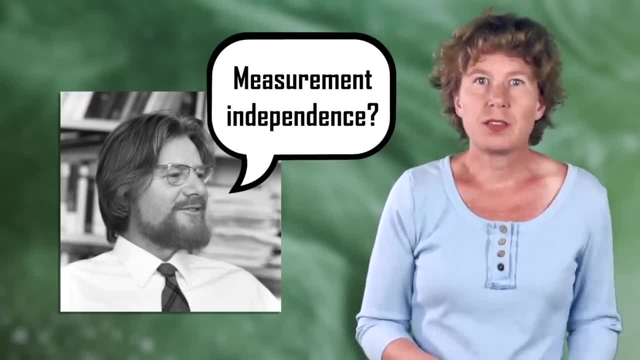 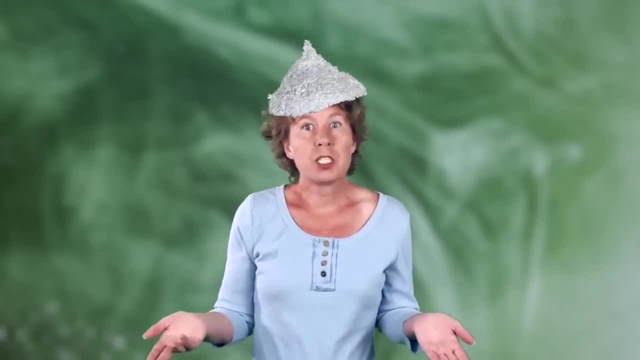 Indeed, most physicists still seem to believe this. At this point. you might think Sabine is talking complete rubbish, Because if that's right, why doesn't anyone ever mention this? Well, first of all, you don't have to take my 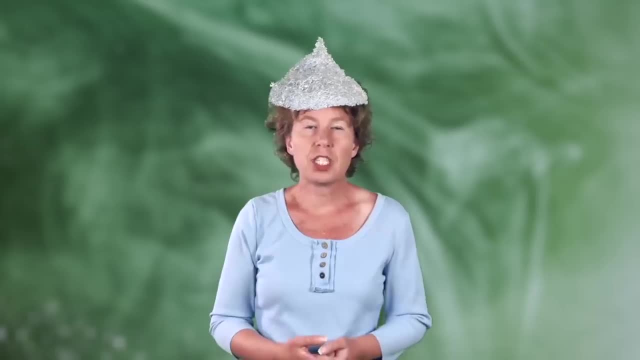 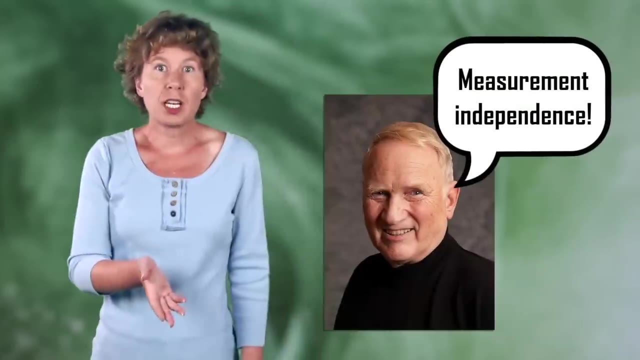 word for it. it's all in the published literature and easy to check. In fact, one of the people who pointed out that Bell had forgotten this assumption was John Bell, John Clauser, who was one of the recipients of the 2022 Nobel Prize. Why physicists refuse? to mention. it is a very interesting question to which I don't have an answer. My best guess is that they want reality to be weird because they like the mystery. There are several hidden variables, models that are local and that reproduce the predictions of quantum mechanics by violating measurement independence. I'll leave you links in the info below. And yes, a violation of measurement independence is a very common problem in the world of quantum mechanics, But it's not just the case. There are also several hidden variables, models that are local and that reproduce the predictions of quantum mechanics by violating 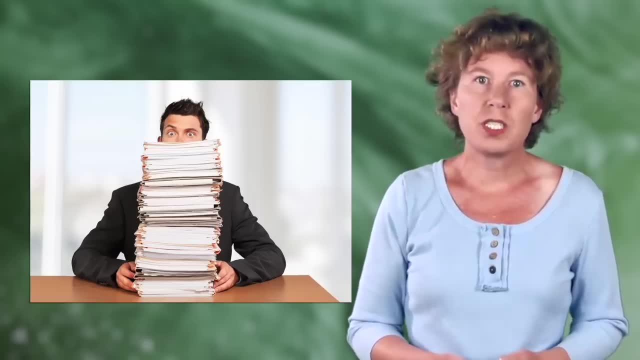 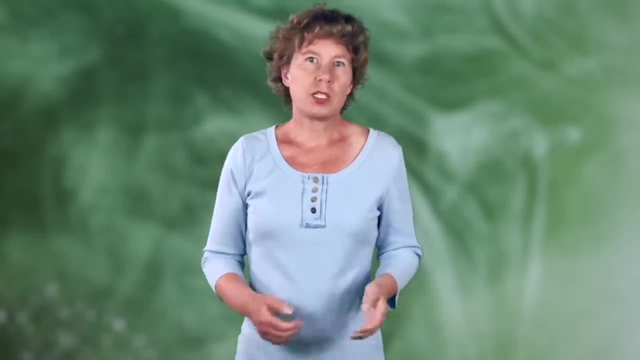 measurement independence. I'll leave you links in the info below. And yes, a violation of measurement independence has also been called superdeterminism, though this term is extremely misleading. I talked about this in an earlier video. In summary, quantum mechanics is not local. 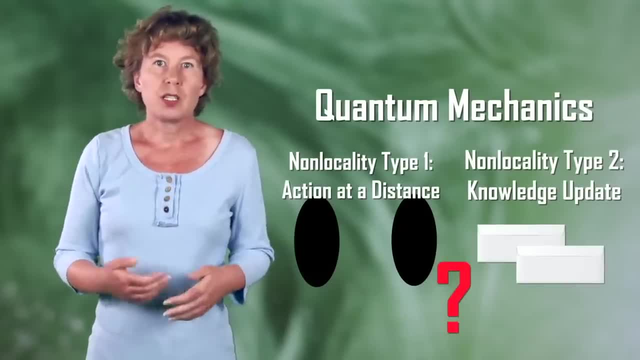 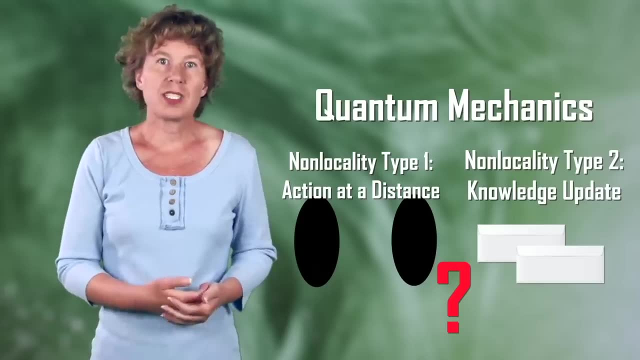 What makes it non-local is the collapse of the wave function. The question is whether this non-locality is physically real. If the collapse of the wave function was a physical process, it would be what Einstein called a spooky action at a distance, and reality would be non-local It. 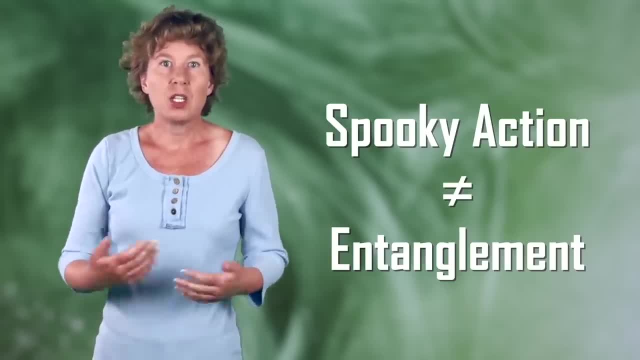 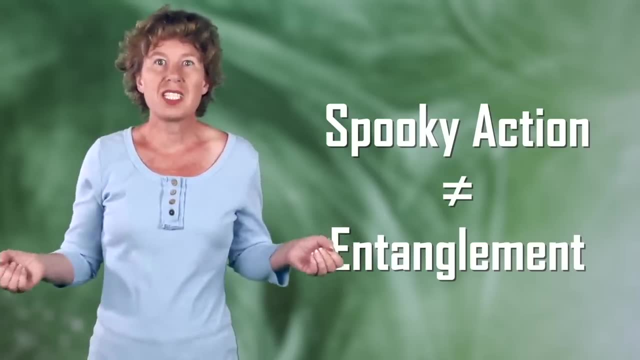 has not been shown that this is indeed the case, no matter how many headlines say otherwise. Entanglement is a non-local correlation that can stretch over long distances, but it's not what Einstein meant by action at a distance, because there's no action in it. 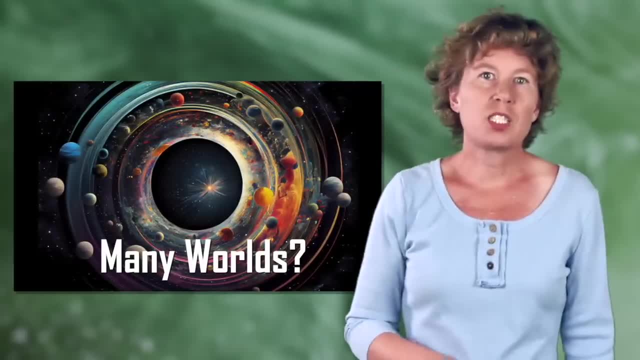 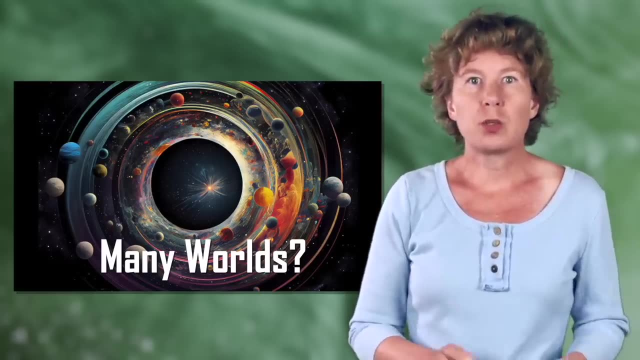 If you're a fan of the many worlds interpretation of quantum mechanics, you probably took issue with some things I said, But this video is already too long, so I'll talk about this some other time. If you want to hear me complain about many worlds, don't forget to subscribe. 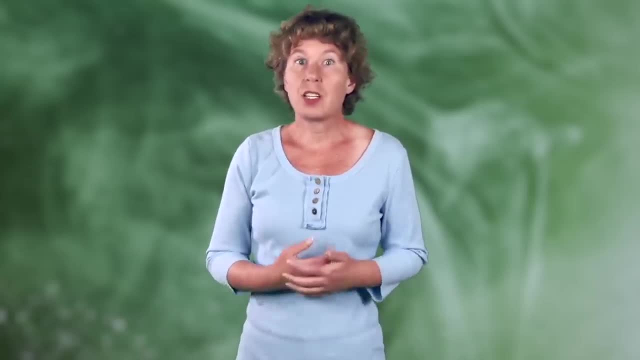 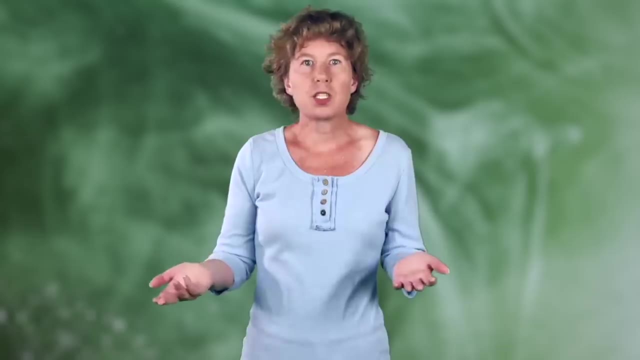 Yes, I admit there's a lot going on in this video that I only touched on very briefly. What is a wave function? how do you get probabilities out of it, how does interference work and why is it important, If you want to understand this? 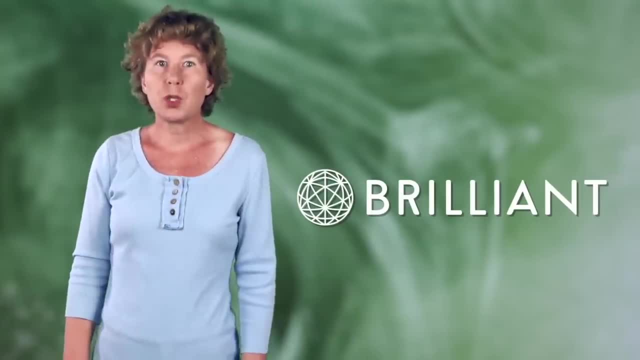 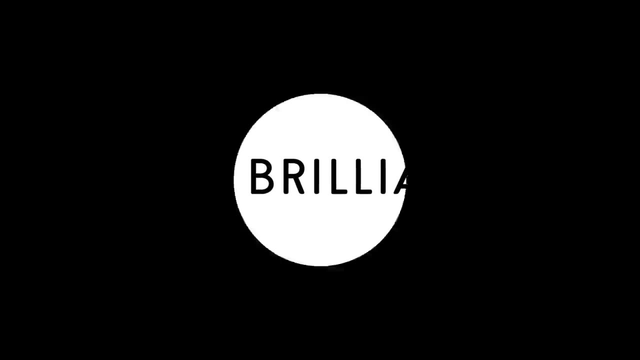 in more depth. you can do this with my course on quantum mechanics at Brilliantorg, who have been sponsoring this video. Brilliant offers courses on a large variety of subjects in science and technology. If you want to learn more about quantum mechanics and quantum mechanics. 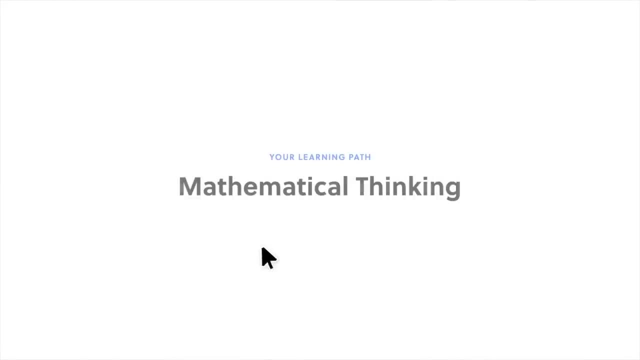 you can check out their website at wwwquantumechanicscom. The great thing about their courses is that they are all interactive with visualizations and follow-up questions, so you can check your understanding right away. This is why I like to look things up on Brilliant. 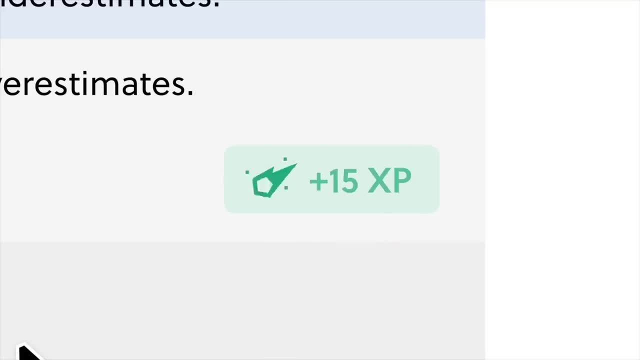 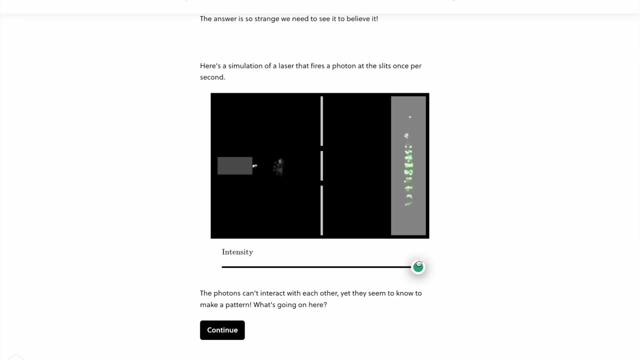 It's fast, it's easy and it tells me what I need to know. My course on quantum mechanics gives you an introduction to interference, superpositions and entanglement, the uncertainty principle and Baal's theorem. It begins from the 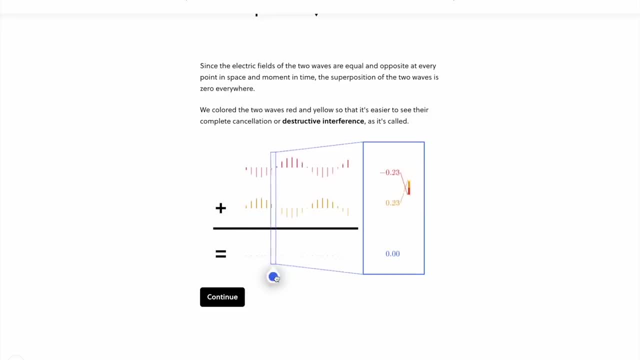 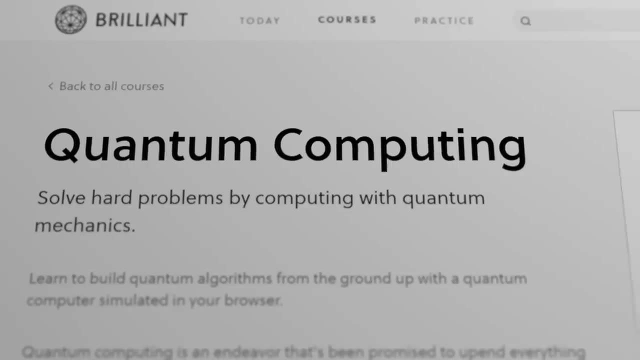 very basics of quantum mechanics, which are the basic principles of quantum mechanics and the basics, so you don't need to bring any background knowledge And after that you can continue, maybe with their course on quantum objects or quantum computing or wherever your curiosity drives you. 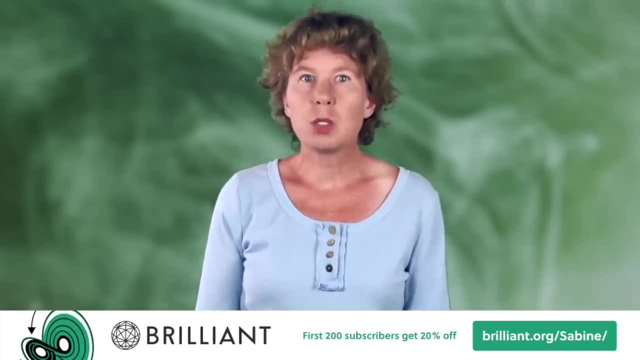 If you're interested in trying Brilliant out, use our link, Brilliantorg- slash Sabine and sign up for a free trial where you'll get to try out everything Brilliant has to offer for 30 days. The first 200 subscribers using this link will also get 20 percent off the 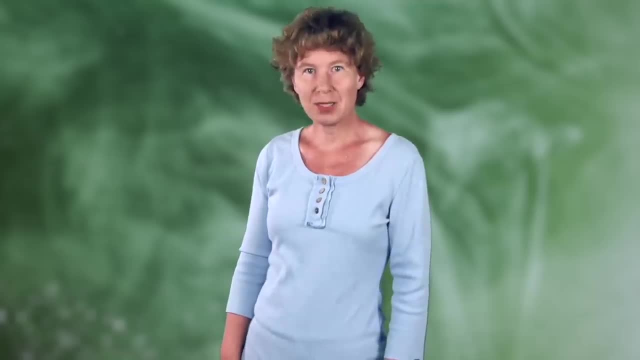 annual premium subscription. Thanks for watching. see you next week.